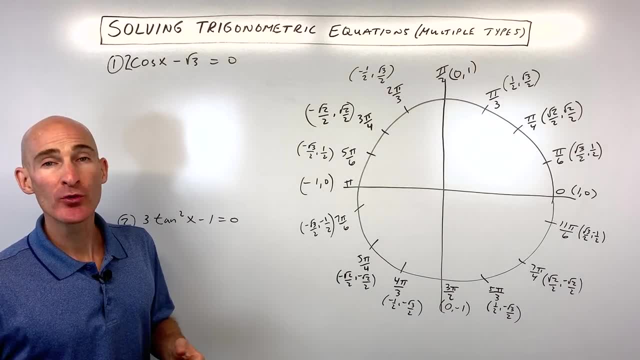 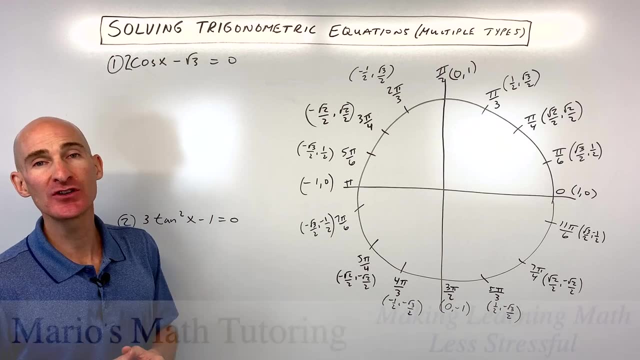 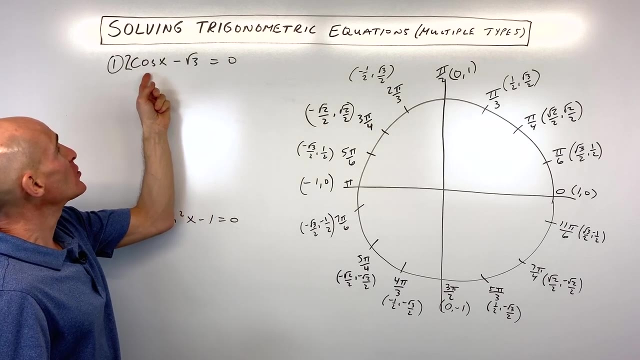 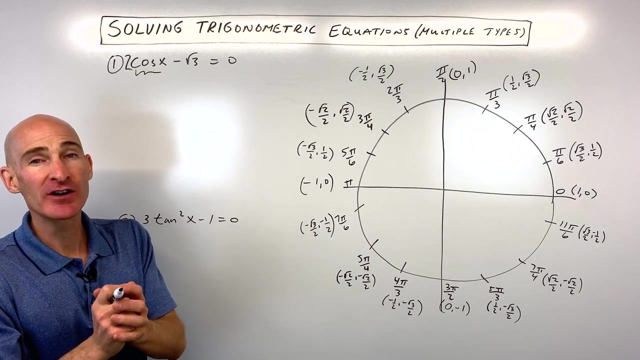 In this video you're going to learn how to solve trigonometric equations. We're going to talk about how to write a general solution, as well as from 0 to 2 pi. We're going to go through 8 examples. Go ahead and pause the video and see if you can do these on your own and we'll go through them together. The first one: we're going to start off easy and get progressively more challenging. It's 2 cosine x minus square root of 3 equals 0.. Now, when you solve these equations, what you want to do is you want to focus on getting that trig function by itself on one side of the equal sign. So let's go ahead and do that by adding: square root of 3 equals 0.. 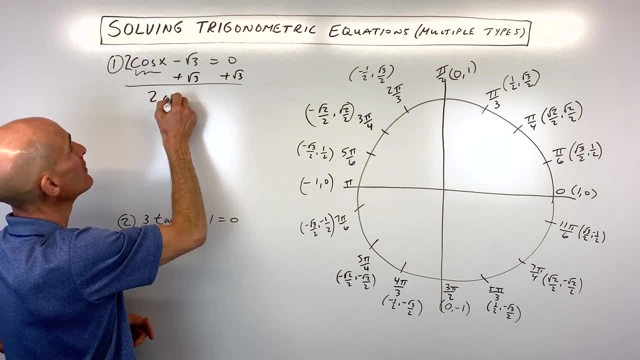 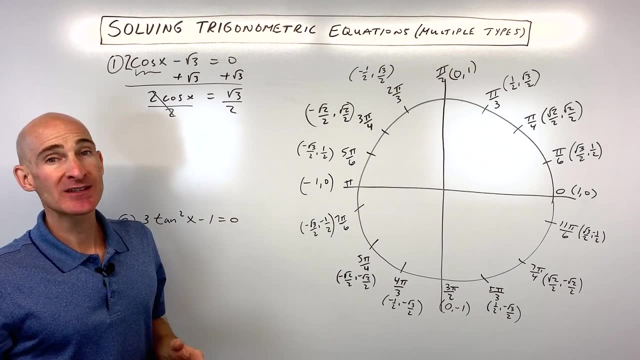 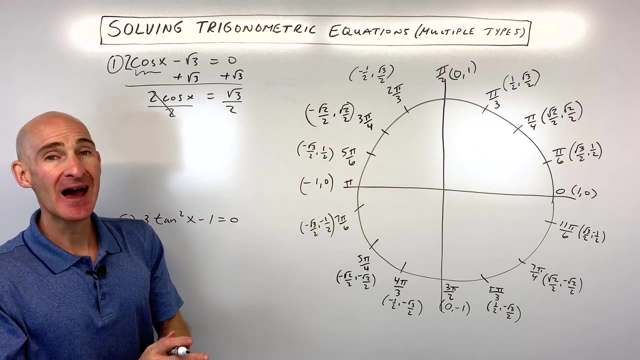 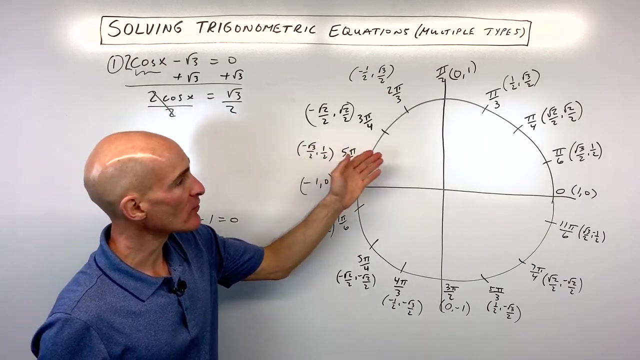 We're going to add square root of 3 to both sides, just like solving an algebra equation, It's just with trig functions. Now what we're going to do is we're going to divide both sides by 2 to get the cosine by itself. So now we're asking ourselves: where is cosine equal to square root of 3 over 2?? Remember, on the unit circle, cosine is going to be the x coordinate, sine is going to be the y coordinate and tangent is going to be y divided by x. So we ask ourselves: where is x square root of 3 over 2?? We can see it's here at pi over 6.. It's also over here at: 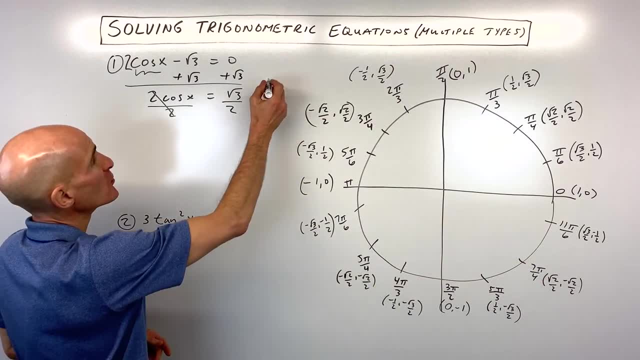 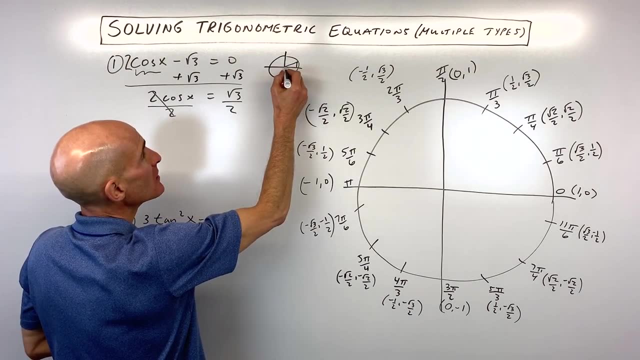 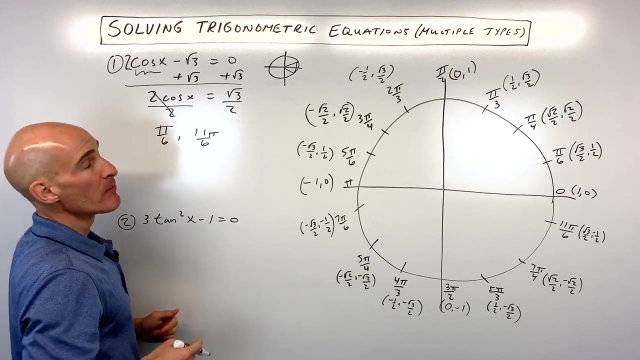 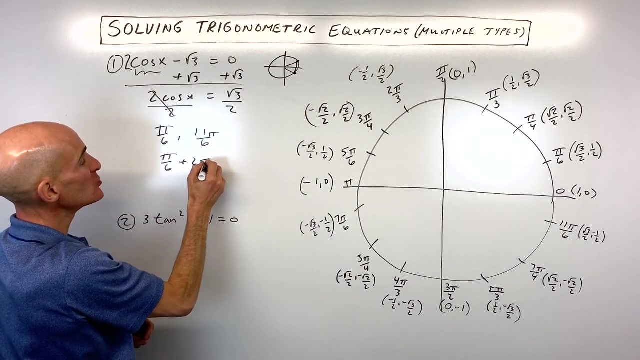 11 pi over 6.. Sometimes what I like to do when I'm doing these problems is I like to make a little sketch for myself, just on the side of the paper, just so I can kind of see what's happening. So I know it's here and I know it's here. So what I'm going to do is I'm going to write this as pi over 6 and 11 pi over 6.. But if we want to write a general solution- see at this point here and this point here- what we can do is we can say pi over 6 plus 2 pi n, meaning that if we add multiples of 2 pi, we're going to end up at that same point on the circle. 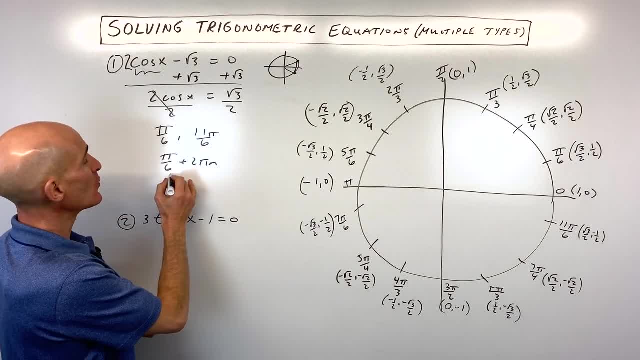 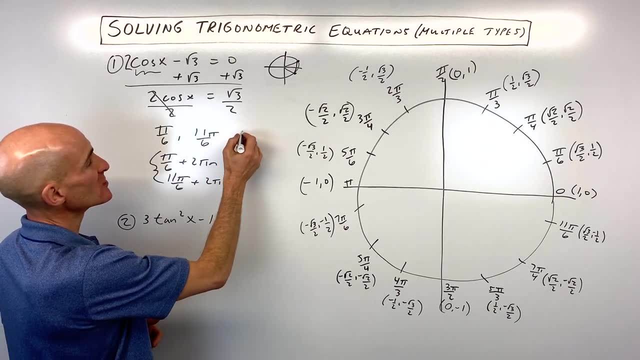 And the cosine value is going to be square root of 3 over 2. there Same thing with 11 pi over 6.. So we can say 11 pi over 6 plus 2 pi n. So this is our general solution. This is our solution. if it just says from 0 to 2 pi, And you got it. 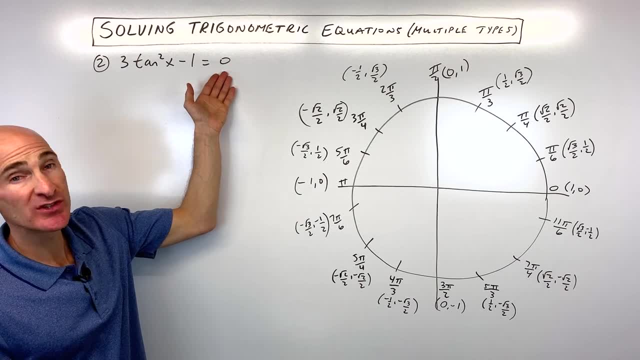 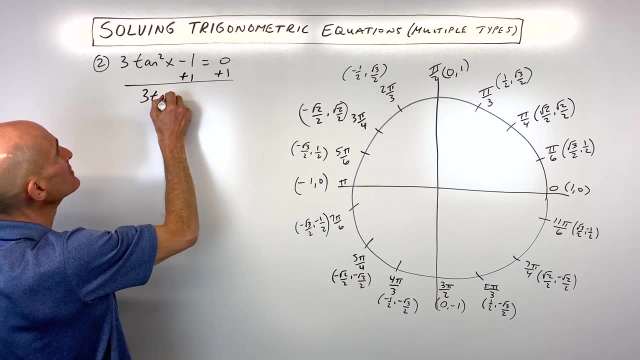 So for number 2, we've got 3 tangent squared x minus 1 equals 0. We want to get that tangent by itself, So let's go ahead and add 1 to both sides of the equation. We've got 3 tangent squared of x equals 1.. Let's go ahead and divide both sides by 3.. We're trying to get that tangent by itself. 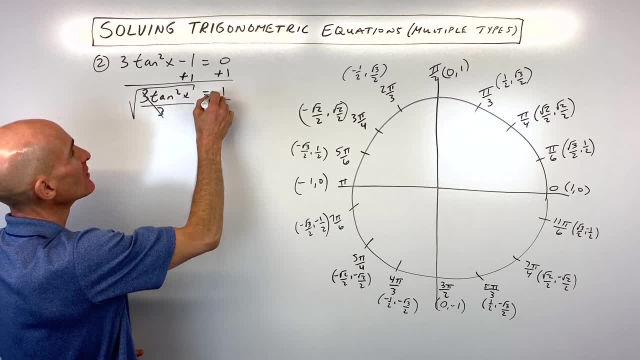 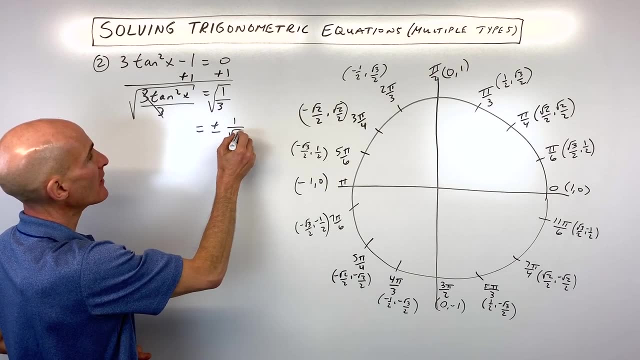 And now what we're going to do is we're going to take the square root of both sides of the equation. Remember, when you do that, you get two answers, Plus or minus: square root of 1, which is 1.. And then here we have square root of 3.. So that's what tangent of x equals. 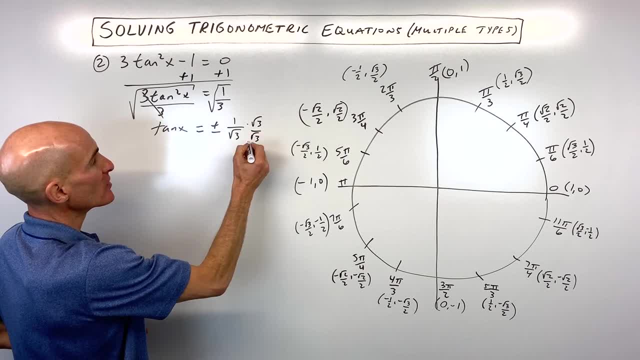 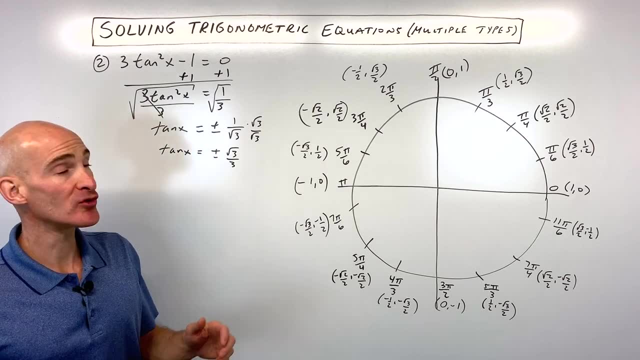 You can rationalize this by multiplying the top and bottom by square root of 3.. So that would give us plus or minus square root of 3 over 3 equals tangent of x. Now remember, on the unit circle tangent is the y coordinate divided by the x coordinate. So we either need to find out where tangent equals. 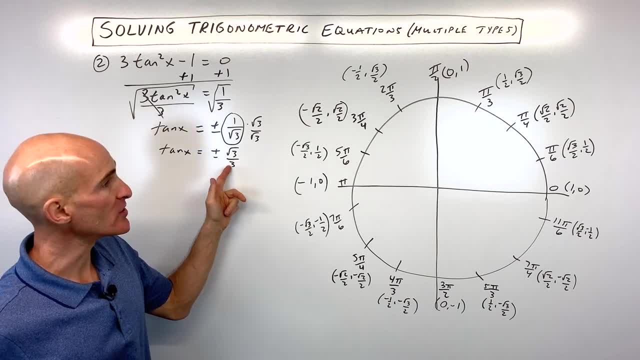 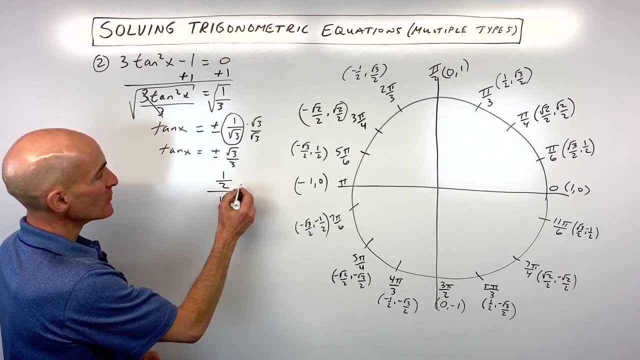 1 over root 3 or, if you rationalize it, square root of 3 over 3.. So y over x. You can see here 1 half divided by square root of 3 over 2.. See if you multiply the numerator and the denominator by 2. See how those 2's cancel and you get 1 over square root of 3.. 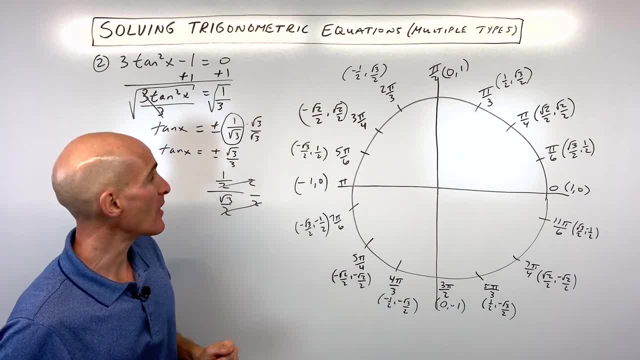 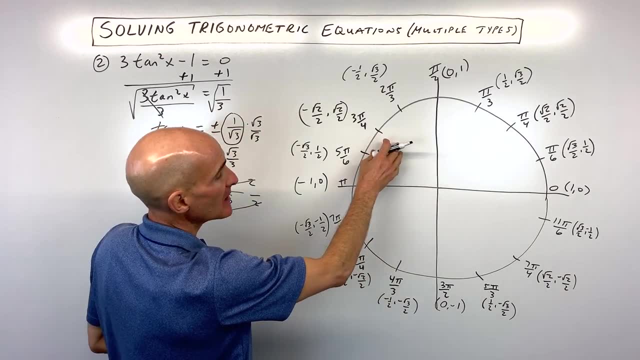 So we know it's a pi over 6 or 30 degree reference angle And you can see it's positive or negative. Tangent is positive in the first quadrant and the third quadrant. Negative in the second and fourth Because in the second quadrant the x's. 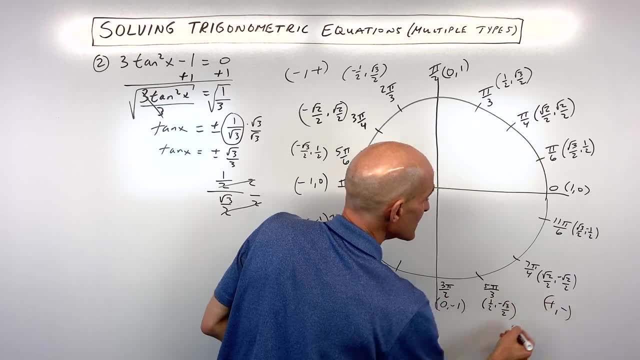 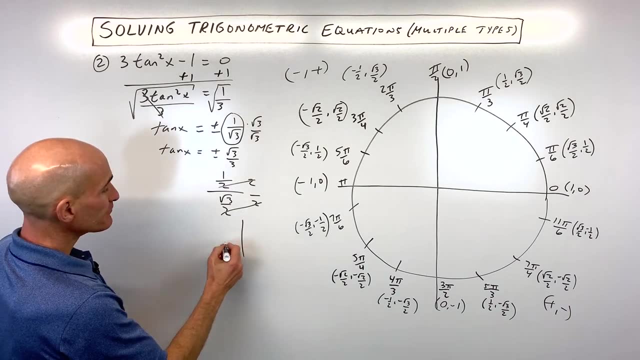 Negative and the y is positive. In the third quadrant it's the reverse: The x is positive and the y is negative. So y over x is going to give us a negative. So here what we can see. I like to draw a little sketch here. We can see it's occurring over here at these 30 degree reference angles. 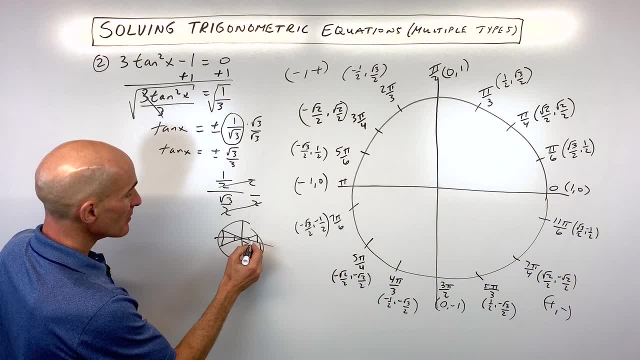 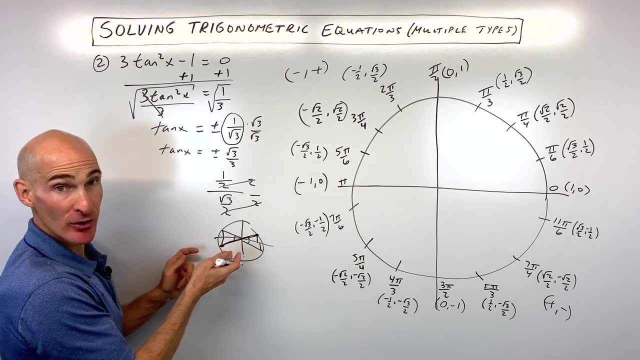 30 degrees, 30 degrees, 30 degrees and 30 degrees. But what's interesting is you see how these points right here are diametrically opposed Meaning like a diameter. Same thing with these 2 points. See how they're across from each other like a diameter. 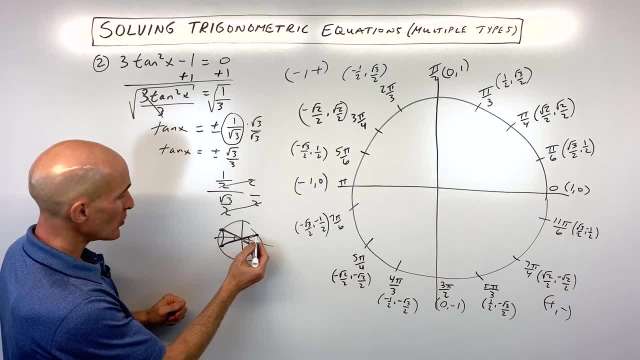 What we can do is we can group them together, And we can group those together when we write our general solution. So let's go ahead and start off with pi over 6.. Okay, so we're going to say x equals pi over 6 plus pi n, this time. 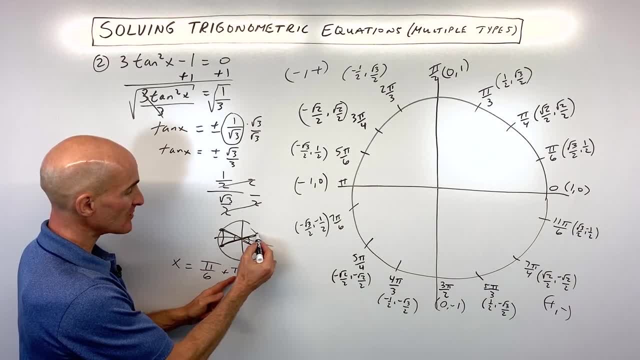 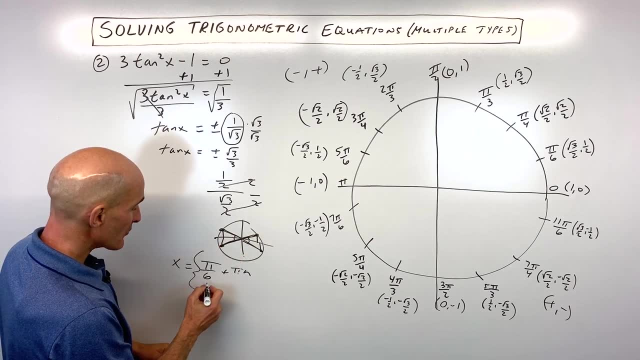 Pi, because we're just adding 180 degrees. If we add another 180 we're back to this point, etc. See, we're always going halfway around the circle And you can also say 5 pi over 6 plus pi n, And so that will take care of these 2 and those 2 and we've gotten all of them. 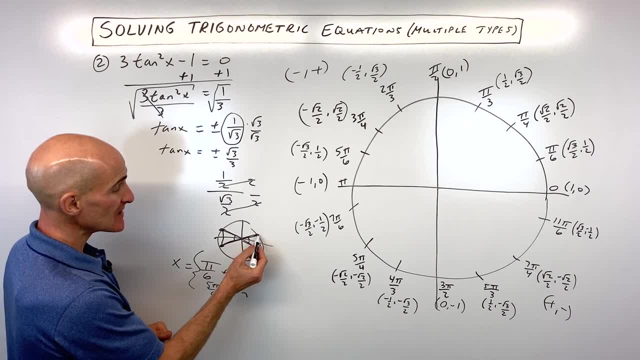 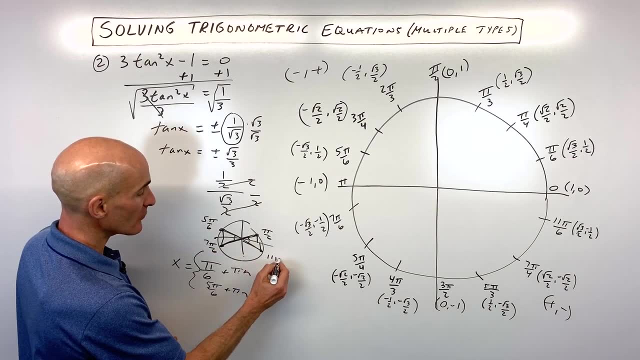 If it just asks from 0 to 2 pi, then you would just list these individually: Pi over 6,, 5 pi over 6,, 7 pi over 6, and 11 pi over 6, and those would be your 4 answers. but this is your general solution. 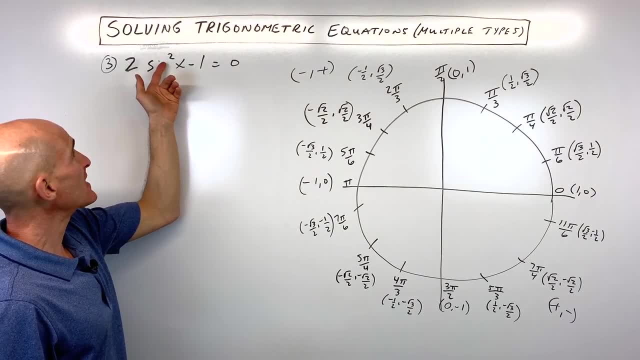 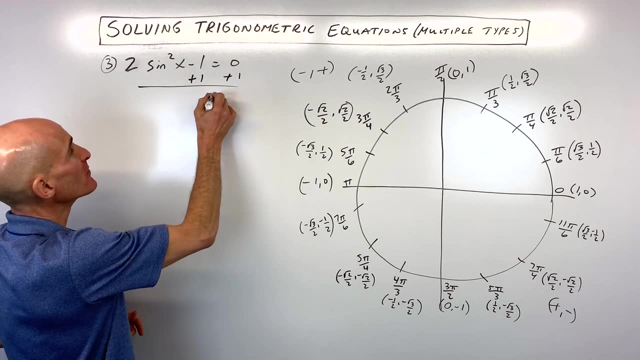 Okay, number 3, see if you can do this one. We've got 2 sine squared. x minus 1 equals 0.. Each one of these problems that I'm doing in this video is a little bit different, because I want you to learn something new each time. 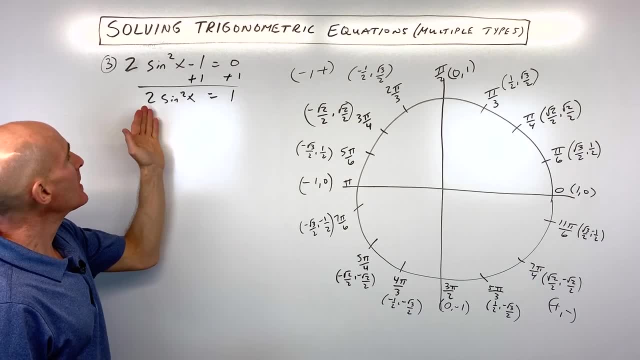 So I'm not going to be repeating like the exact same type of problems. I want to show you something unique. So here what we're going to do is we're trying to get that sine by 1.. I'm dividing both sides here by 2.. 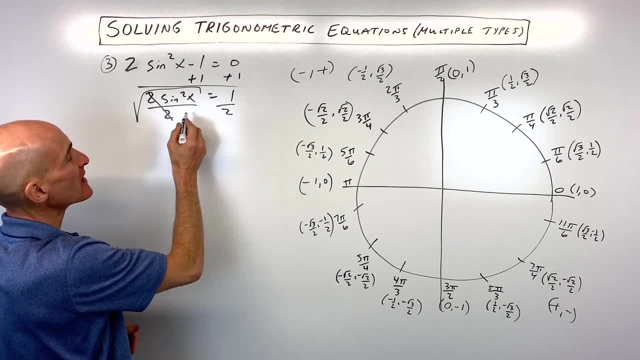 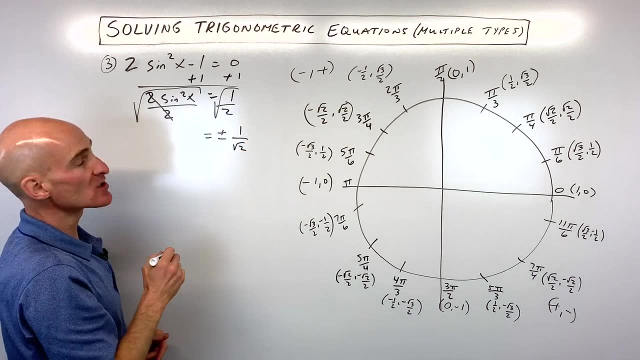 And then we want to take the square root to get rid of that sine squared there. We want to do the inverse. When we do that, we get 2 answers Plus or minus: square root of 1, which is 1.. Square root of 2, which is square root of 2.. 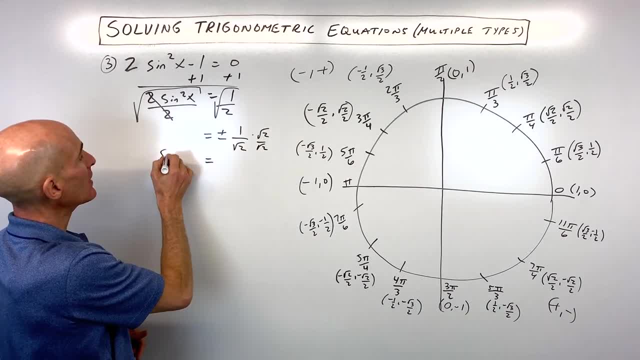 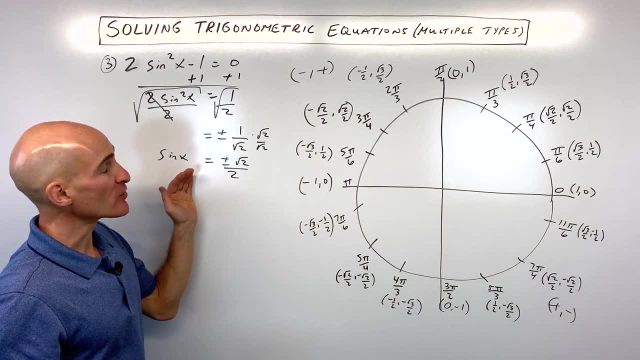 If we rationalize by multiplying top and bottom by square root of 2. We get where is sine of x equal to plus or minus square root of 2 over 2.. So let's take a look Now. remember: sine on the unit circle is the y coordinate. 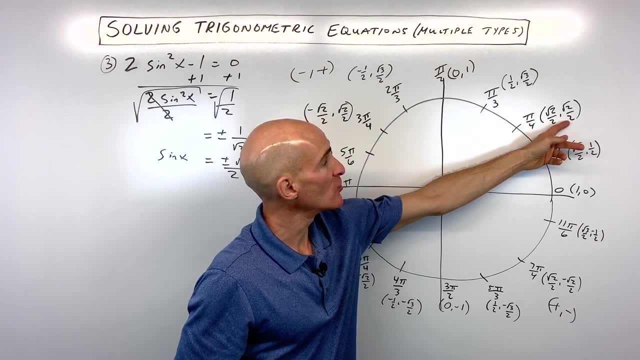 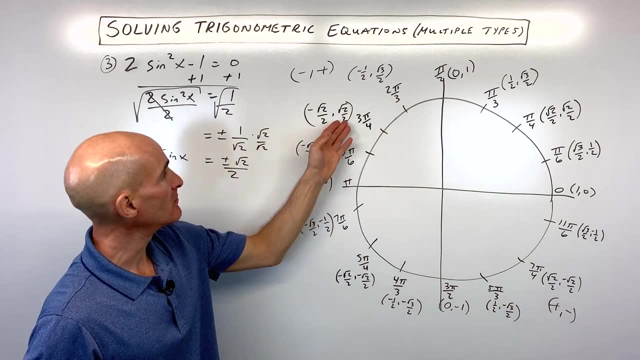 You can see, sine is going to be square root of 2 over 2 over 2.. So we're going to do that. So here, Negative square root of 2 over 2 down here As well as here, And positive square root of 2 over 2 here. 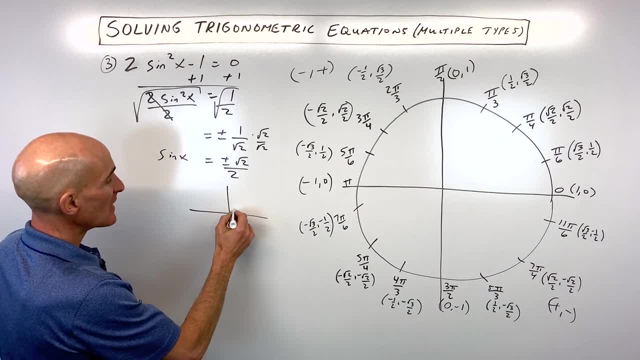 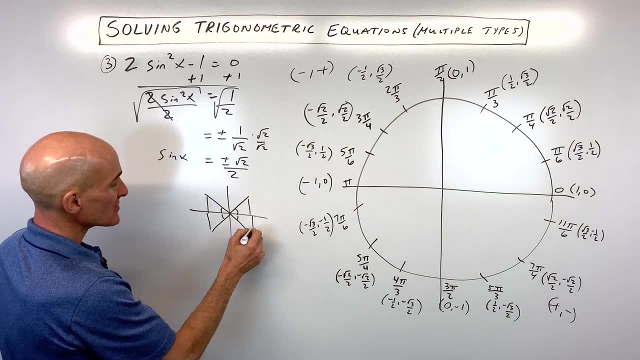 So again I like to draw a little sketch. You can see it's going to be at these 45 degree reference angles, 45 degrees with the x axis. So all these triangles are the same. But what's interesting in this particular problem is 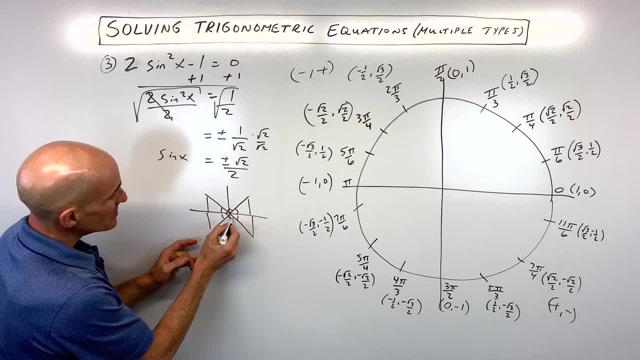 I don't know if you can see this, But see how these are at right angles to one another, Meaning they're 90 degrees apart. So what I can do is I can group them together, I can say at pi over 4.. 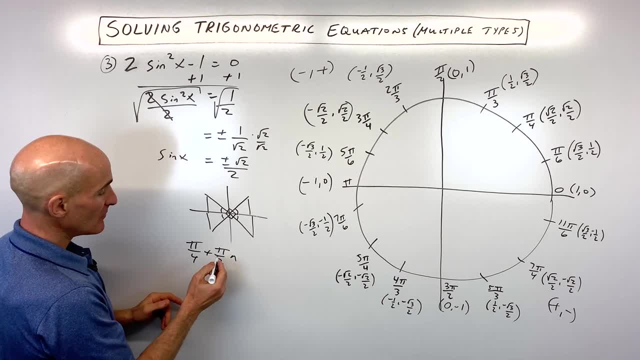 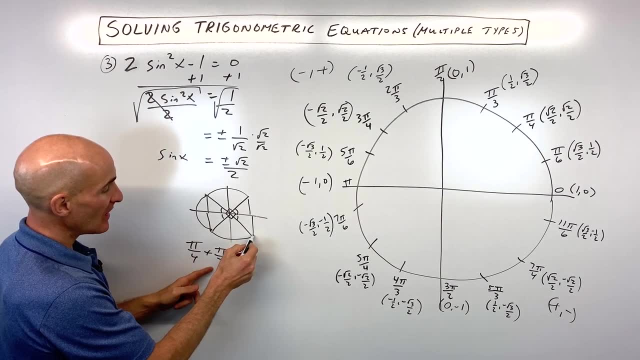 If I add multiples of 90. Meaning pi over 2 in radians, Pi over 2n. So if I add 90, I end up at this point. If I add another 90 at this point, If I add another 90 at this point. 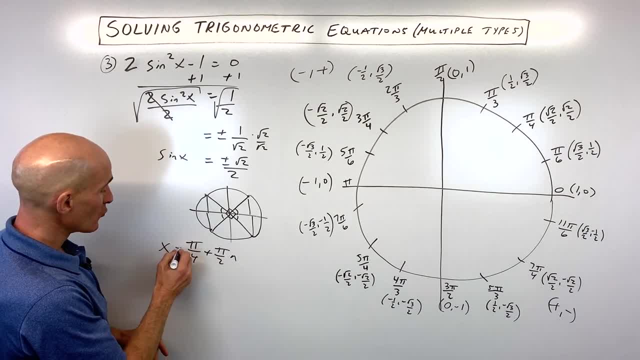 And then I'm back to where I started. So what we can do is group these all together In this one expression here: Pi over 4 plus pi over 2n, That's where sine is going to be positive root 2.. 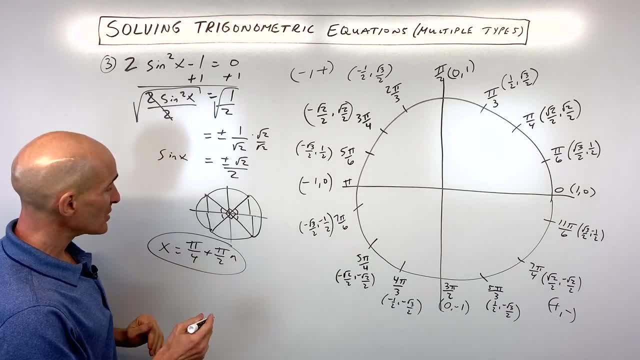 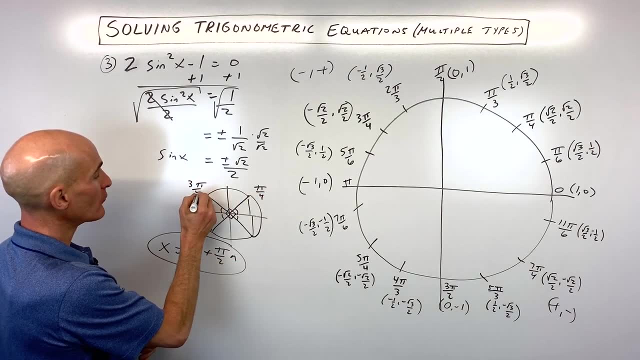 Or negative root, 2 over 2.. If we wanted to just list them, If it just said what's the answer between 0 and 2. And 2 pi, Then we just list them individually: Pi over 4.. 3- pi over 4.. 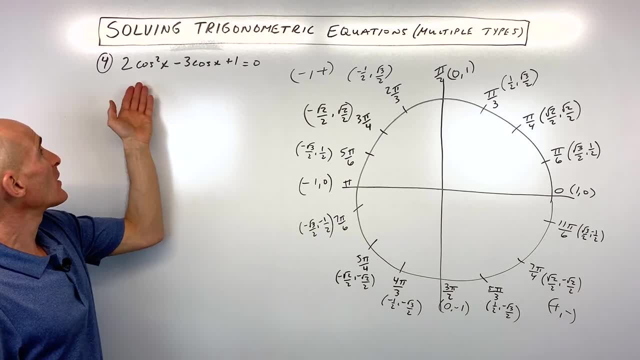 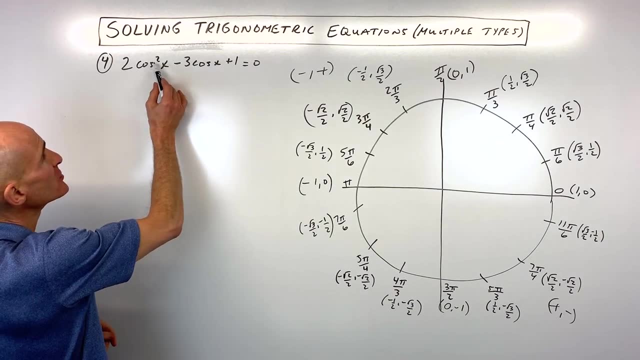 5 pi over 4.. And 7 pi over 4.. And you got it, Number 4.. See if you can do this one. We have 2 cosine squared x minus 3. cosine x plus 1 equals 0.. 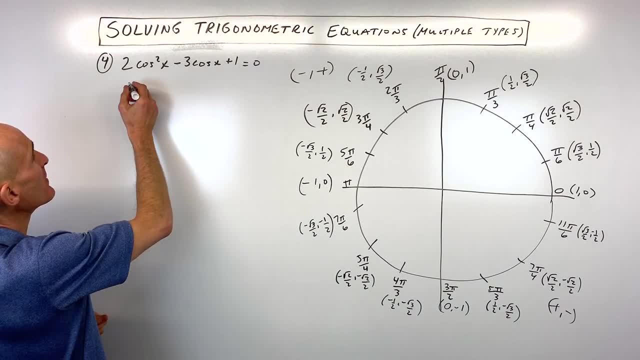 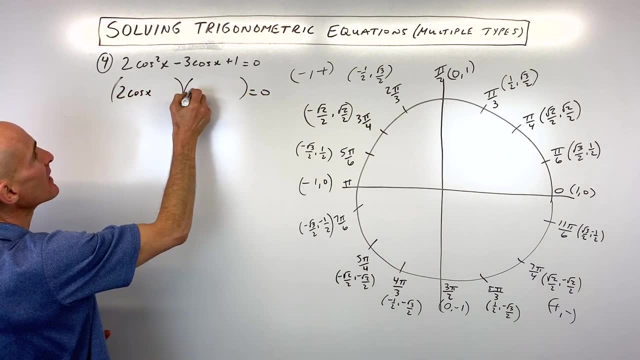 What's interesting about this one Is we have a squared term As well as a cosine to the first term. So what I'm going to do in this one, What we have here, is we have 2 cosine x Times, 1 cosine x. 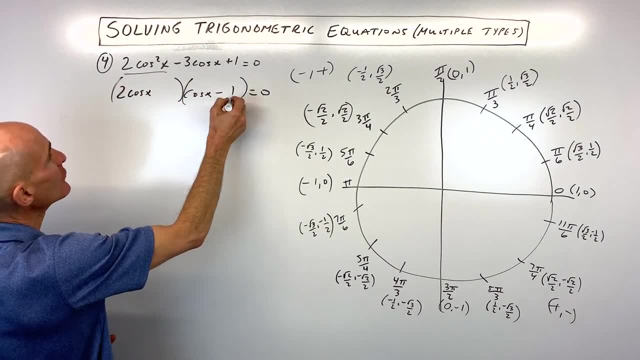 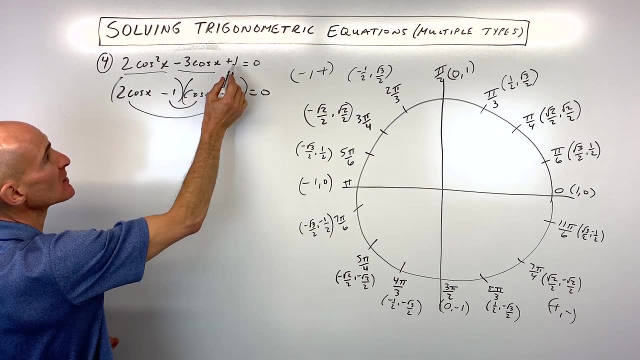 Gives us back the 2 cosine squared x And if I do, negative 1 and negative 1.. This will give us negative cosine x, Negative 2 cosine x, Which adds up to negative 3 cosine x And negative 1 times negative 1 is positive 1.. 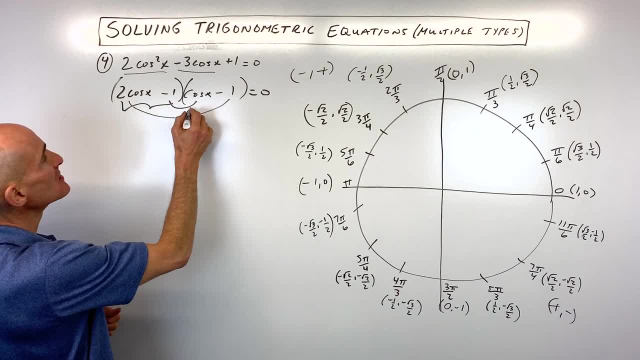 So we just factored it. Now, what we're going to do is we're going to take each of these groups And we're going to set them equal to 0.. Each of these factors- So 2 cosine x minus 1- equals 0.. 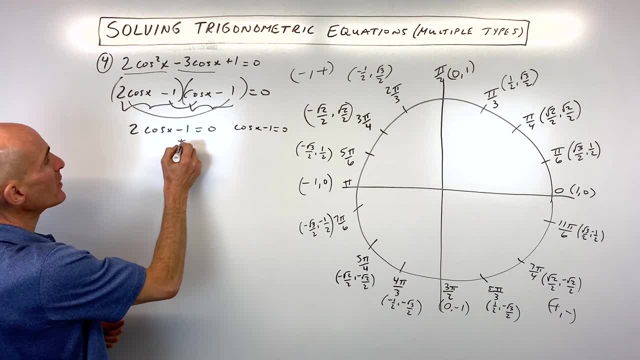 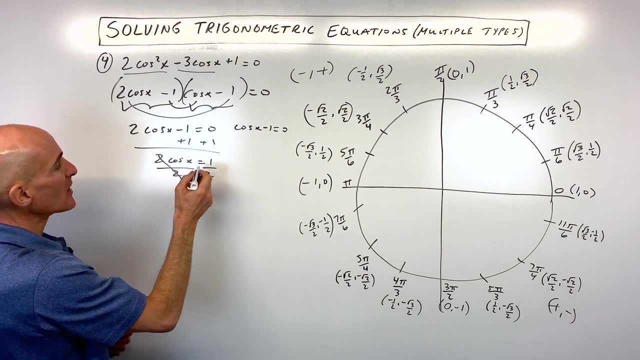 And cosine x minus 1 equals 0.. So if we add 1 to both sides, We've got 2. cosine x equals 1.. Divide both sides by 2.. Okay, so we're looking at Where is cosine equal 1 half. 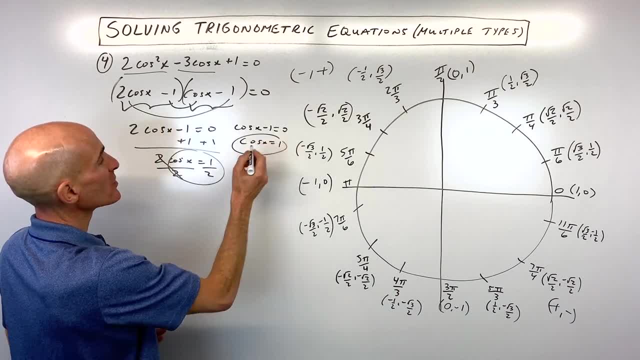 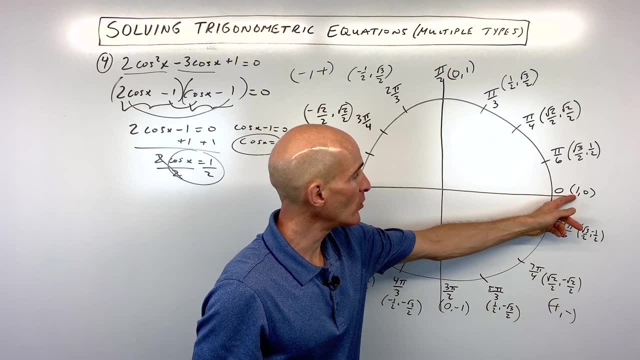 And here, if we add 1 to both sides, We say: where is cosine equal to 1.. So let's look at this one first. So cosine is the x coordinate on the unit circle. Where is x equal to 1.. Well, you can see that's going to be right here at 0. 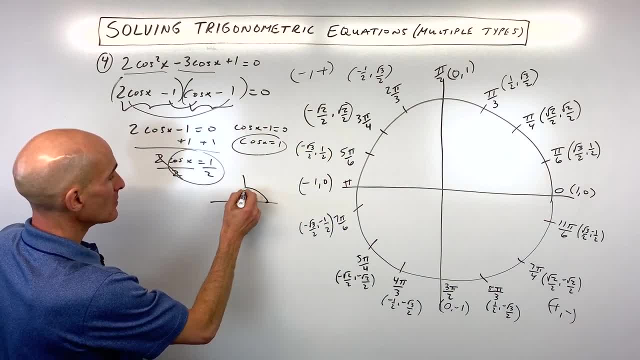 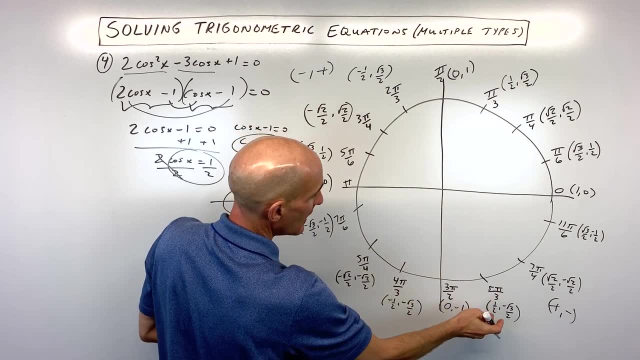 So right here. And then, where is cosine a half? Well, we know, cosine is again the x coordinate on the unit circle. Where is cosine equal to 1. It's going to be a half here at pi over 3.. And also here at 5 pi over 3.. 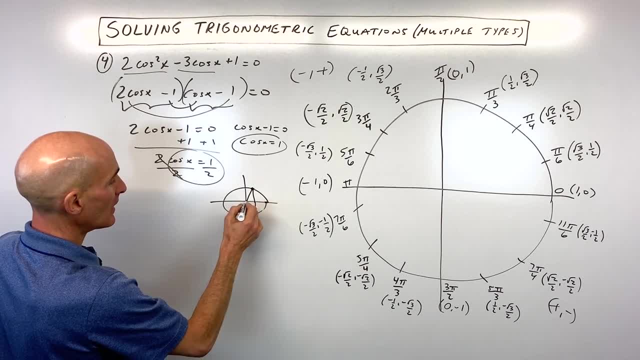 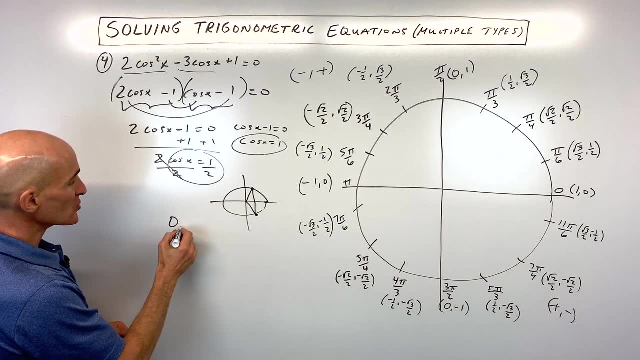 So let's go ahead and sketch that Pi over 3. And 5 pi over 3.. So those are going to be our answers, But let's see what we can do as far as a general solution. So we said 0.. 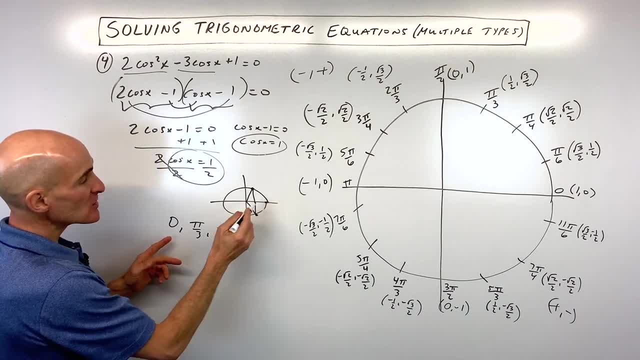 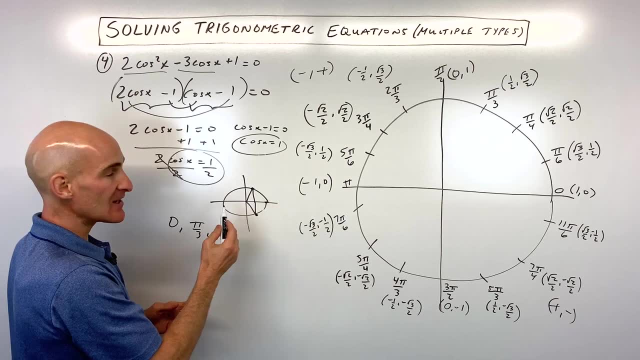 Pi over 3.. 5 pi over 3.. But you can see now these ones, They're not in such a way that if I just add like 180 degrees, I'm at one of the other points, Or if I add 90 degrees, like one of the other questions we did. 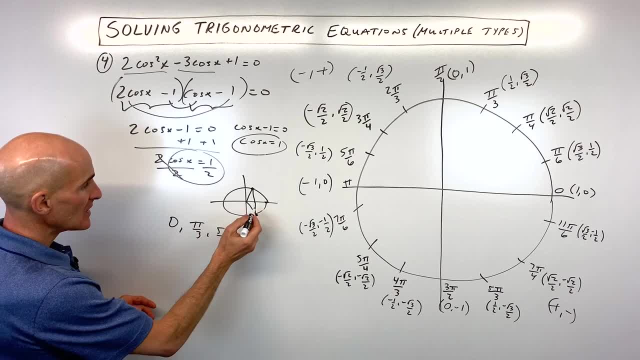 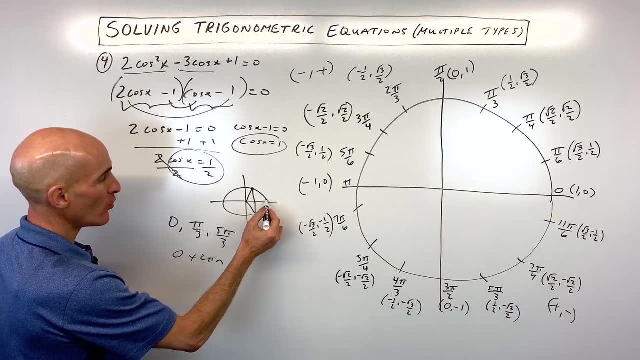 Here what we're going to have to do. We're going to have to do them individually. We're going to have to say 0. Plus 2 pi, n Meaning if I add multiples of 2 pi. I'm going to end up at this point. 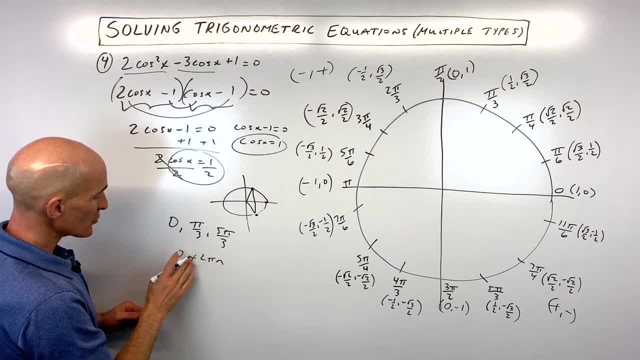 By going around the circle, You know one whole revolution. We don't really need the 0 so much, But I'll just leave it for now. It also could be pi over 3. Which is here, And we can add multiples of 2 pi. 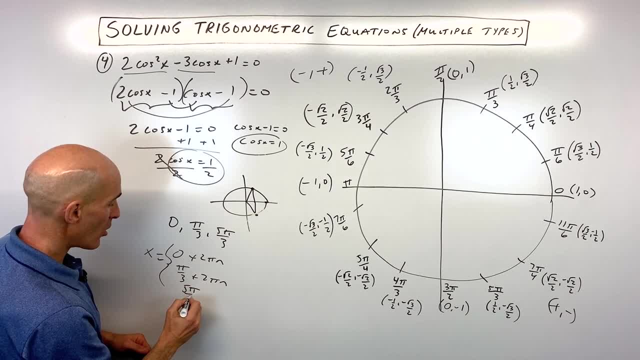 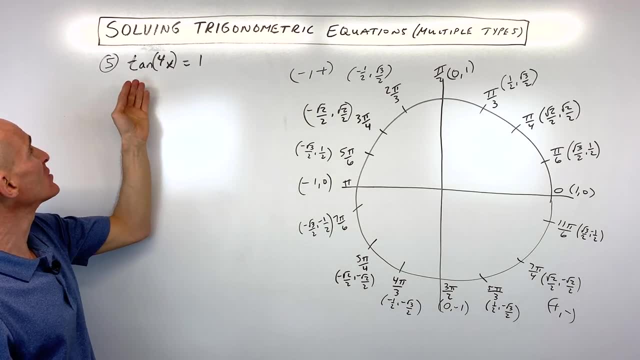 So pi over 3 plus 2 pi n, And then the last one, 5 pi over 3. Number 5. This is referred to as a multiple angle trig equation, Because we've got tangent of not 1x But 4x equals 1.. 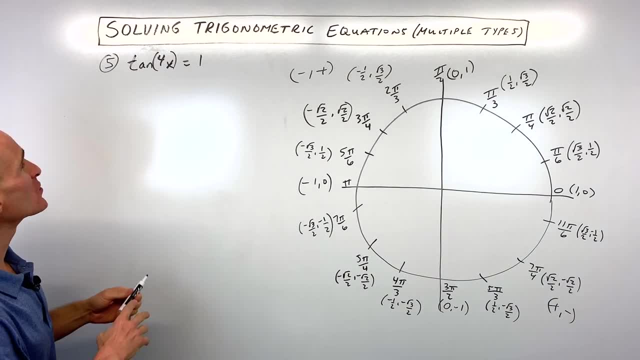 So how would you solve that problem? Well, what we're going to do Is we're going to pretend like this is a group or a chunk. We're going to treat this all like one quantity. So we're going to say: tangent of what angle equals 1.. 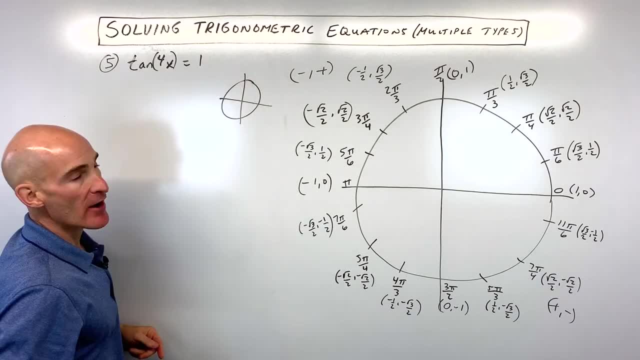 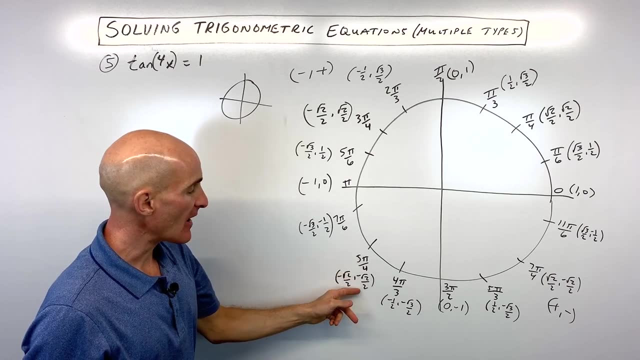 Well, we know, on the unit circle Tangent is y over x. So y divided by x has to equal 1.. And that occurs here at pi over 4.. As well as over here at 5, pi over 4.. Negative divided by a negative is going to give us a positive 1.. 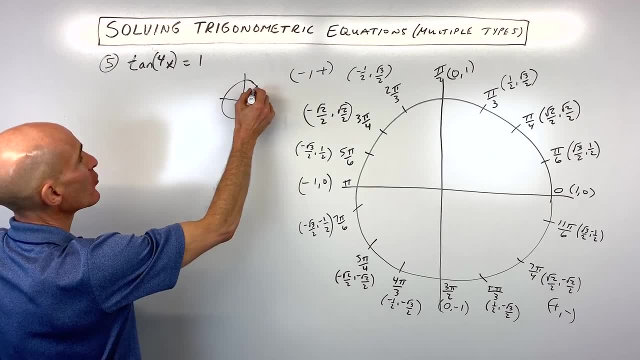 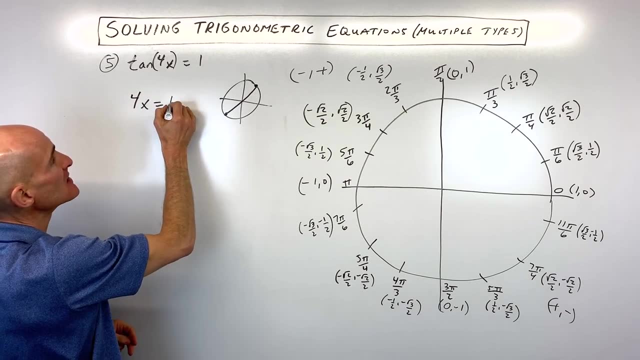 So you can see that these are across from each other Like so. So if we were to write a general solution, We would say 4x, So not x. but 4x Is equal to pi over 4. Plus pi n. 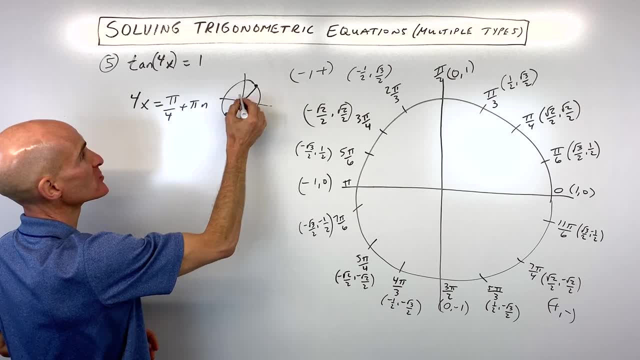 Because we're adding 180 degrees. We're going half way around the circle each time To end up at each one of those points. But we don't want to solve for 4x. We actually want to solve just for 1x. 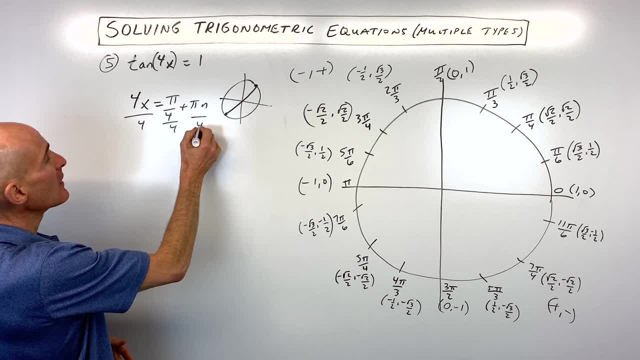 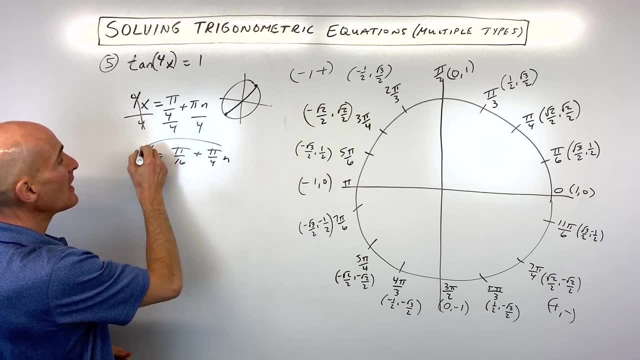 So what I'm going to do is divide everything by 4.. If we do that, That's going to give us x equals pi over 16.. Plus pi over 4 n, And that's our general solution. But if the instructions on your question here say: 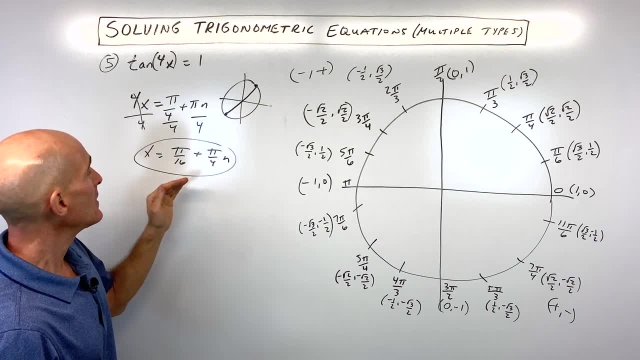 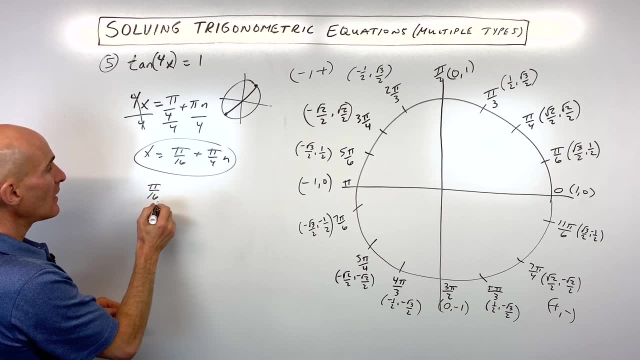 Find all the angles between 0 and 2 pi. What you can do is You can start off by Taking n equals 0. That would give you pi over 16. And pi over 4. Is really like 4 pi over 16.. 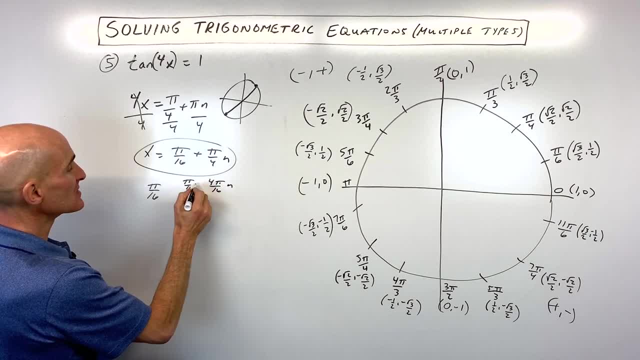 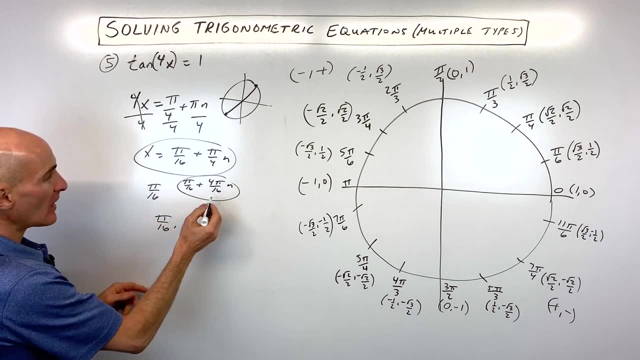 Right. So this is really like pi over 16.. Plus 4 pi over 16 n. So the first angle, If n is 0. Is going to be pi over 16. And if n is 1. That's going to be pi over 16.. 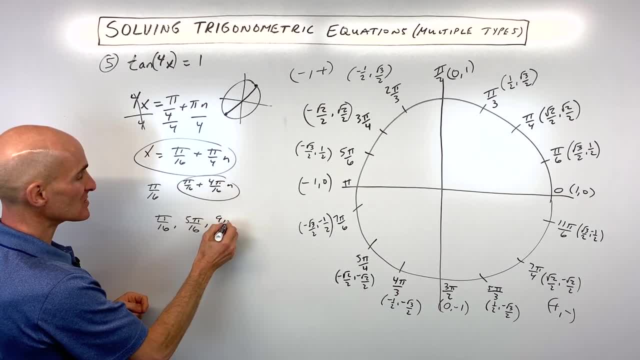 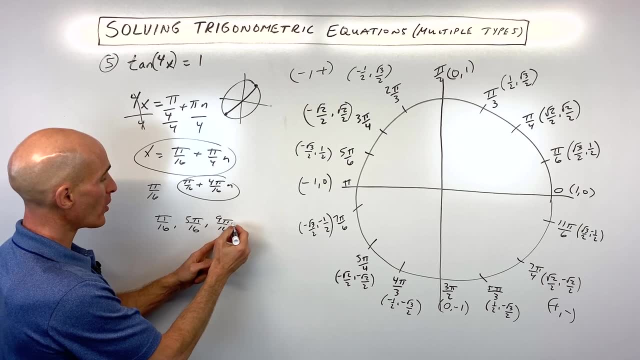 Plus 4 pi over 16. Which is 5 pi over 16.. If n is 2. That's 8 pi over 16.. Plus pi over 16. Which is 9 pi over 16.. And you want to keep going. 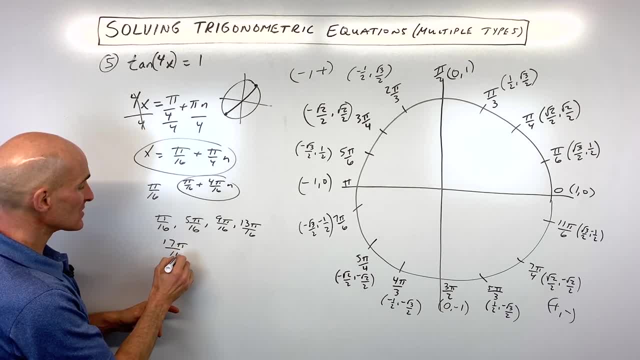 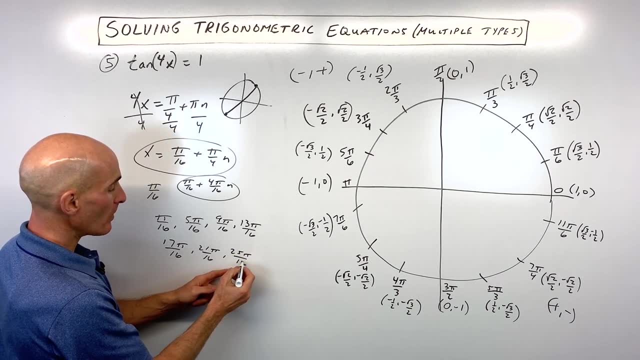 But you don't want to exceed 2 pi, So let's just keep going a few more: 21 pi over 16.. 25 pi over 16.. Now the next one is going to be, Let's see, 29 pi over 16.. 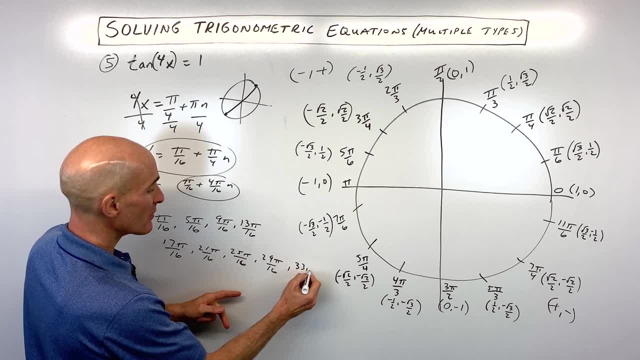 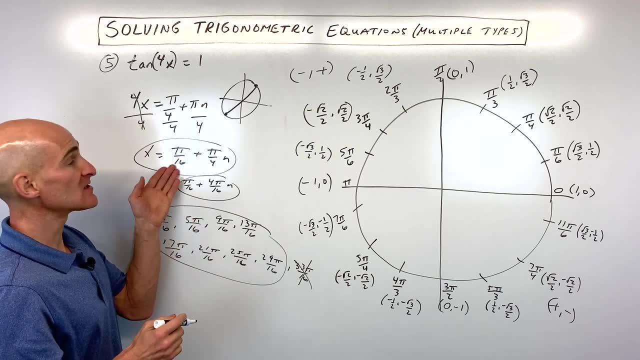 If I go one more, That's going to be 33 pi over 16.. But you can see that's more than 2 pi. So we're going to stop there And these are going to be the answers Between 0 and 2 pi. 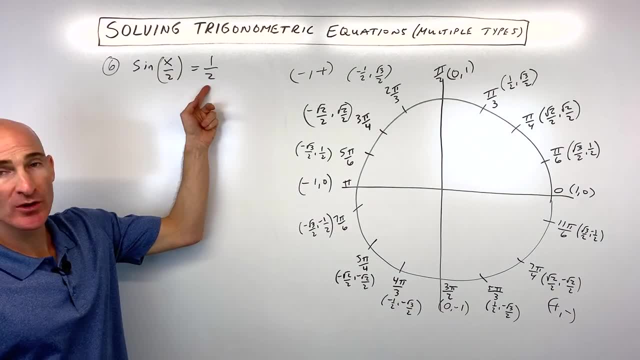 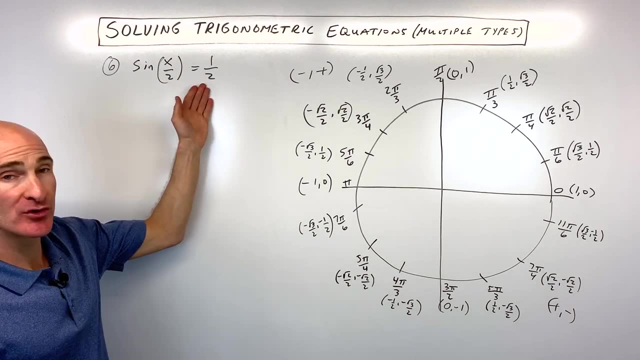 This is going to be your general solution And you got it In number 6 we've got. We think of it as a group. We say: sine of one angle equals 1 half. On the unit circle the sine is the y coordinate. 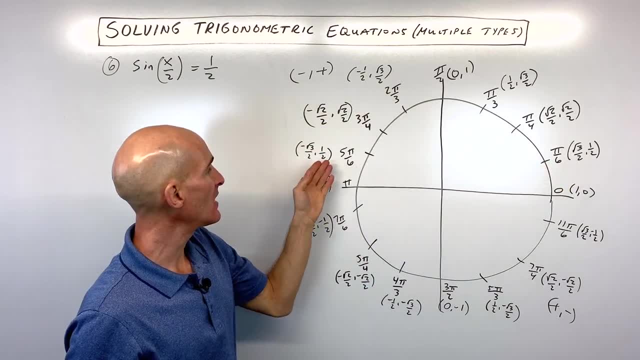 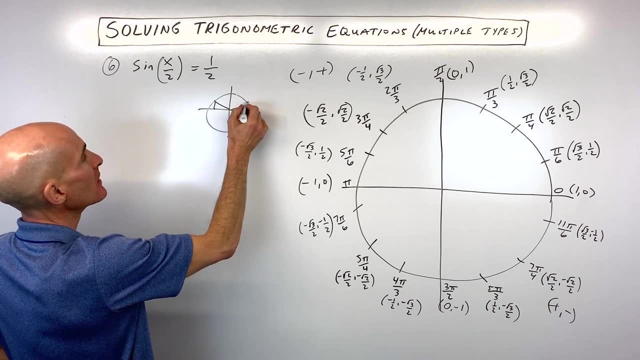 So you can see, sine is going to be a half here At pi over 6. As well as over here at 5 pi over 6.. So let's just draw a diagram. So that's going to be here And here. 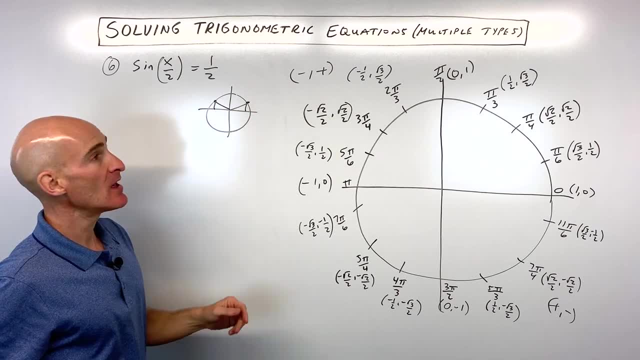 Now you can see they're not really across from each other. They're not adding 90 degrees each time. We're going to have to write these separately. So what I'm going to do is I'm going to say X divided by 2.. 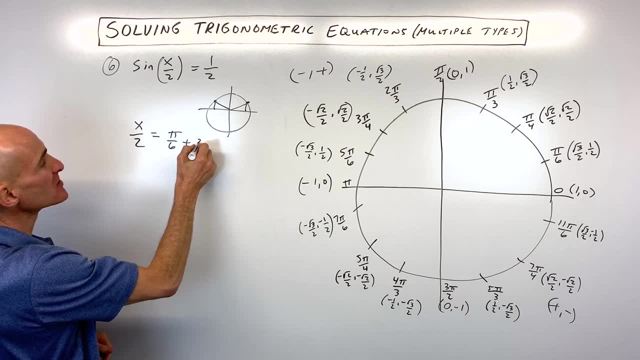 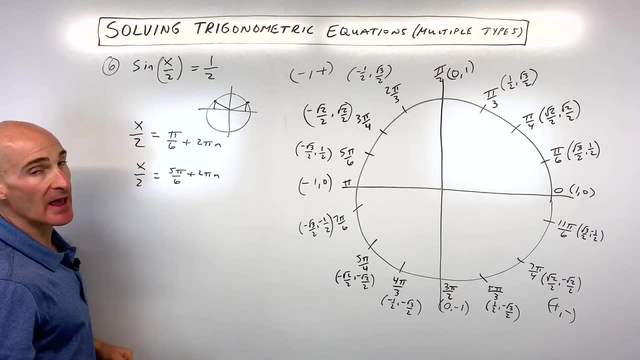 That's the angle. we solve for 5 pi over 6. Plus 2 pi n. And x divided by 2 equals 5 pi over 6. Plus 2 pi n. Now we don't want to solve for x divided by 2.. 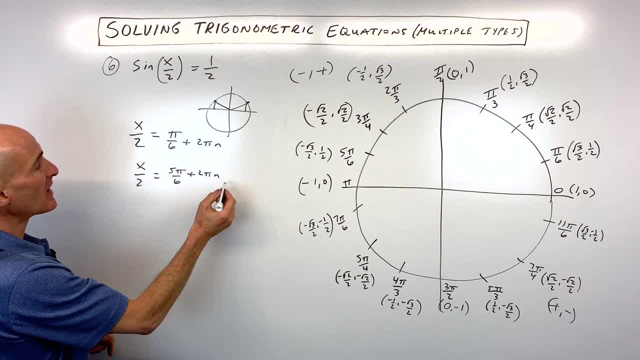 We actually just want to solve for x. So what I'm going to do is I'm going to multiply everything in this equation by 2.. So if we do that, That's going to come out to: x equals 2 pi over 6.. 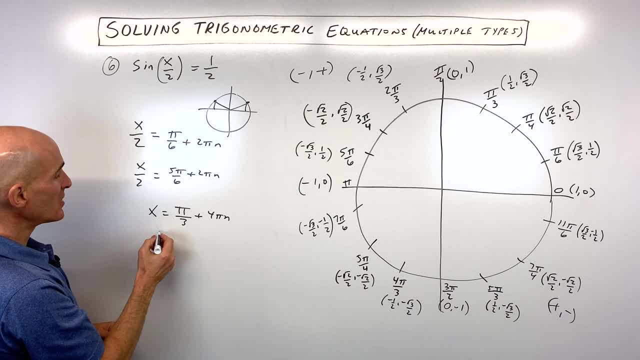 Which reduces to pi over 3. Plus 4 pi n. And if we multiply through by 2 here We're going to get 10 pi over 6. Plus 4 pi n. Now, this is our general solution. But if it just said: 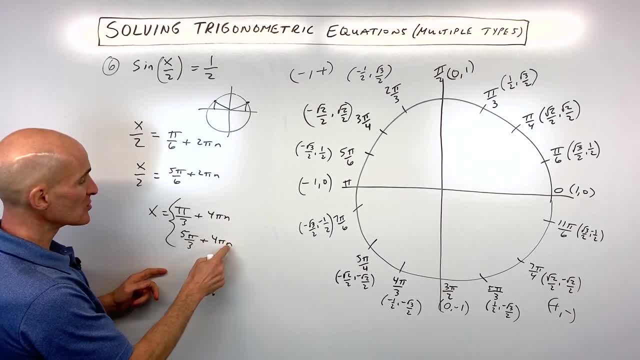 Find all the angles between 0 and 2 pi. What we can do is we can start off by putting in 0 for n. here We're going to get pi over 3.. We're going to get 5 pi over 3.. 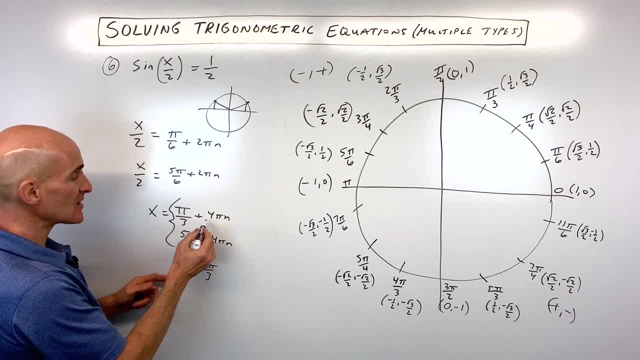 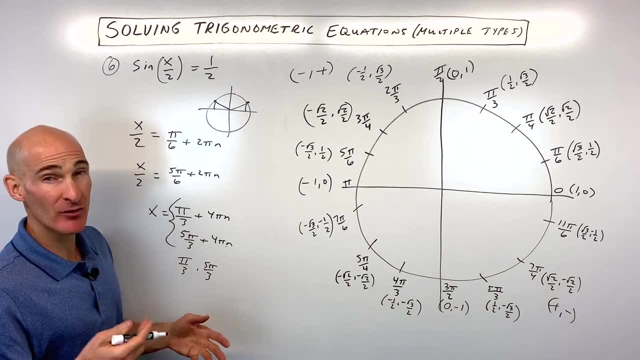 If we make n 1. You can see that's going to be 4 pi Plus pi over 3. Which exceeds our 2 pi. Same thing here if this was 1. This is 4 pi plus 5 pi over 3.. 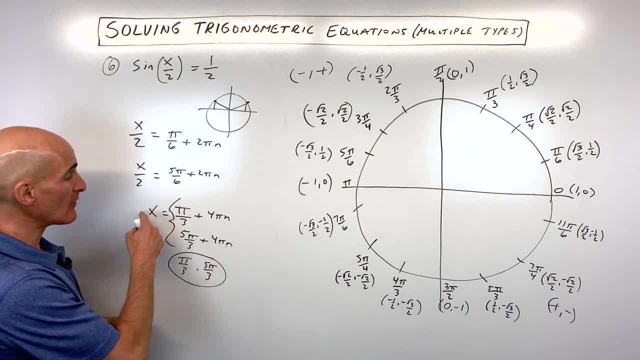 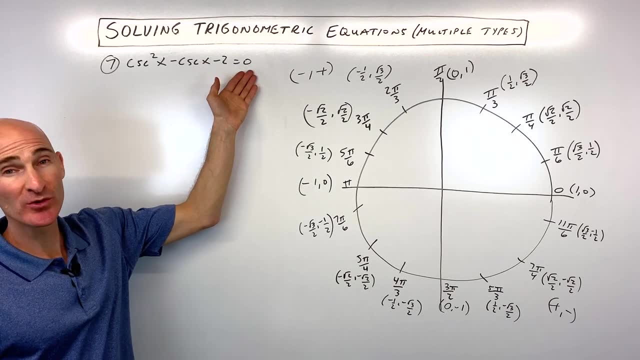 Which exceeds 2 pi. The solution is between 0 and 2 pi, But this here is our general solution. Okay, number 7.. See if you can do this. one Cosecant squared x minus cosecant x minus 2 equals 0.. 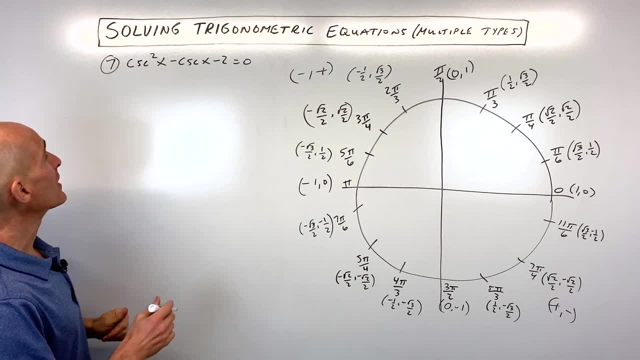 So up to this point we've just been working with sine cosine and tangent. Now we're getting into some of the reciprocal trig functions here, And so the thing I'm going to do with this one- Because I've got a squared term- and cosecant to the first, 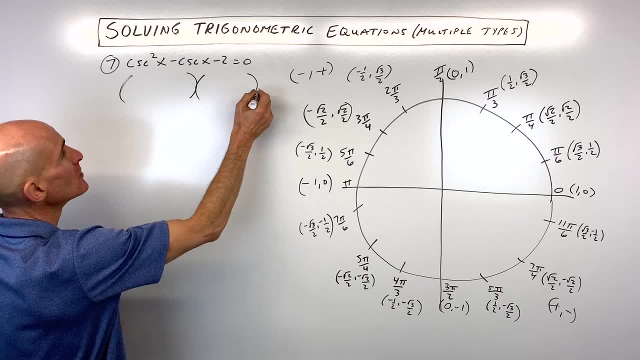 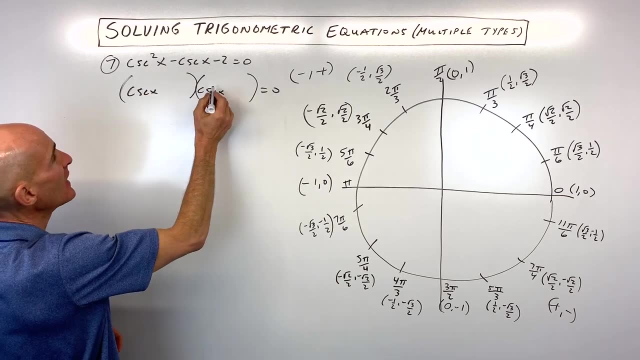 I'm going to factor this Into two binomials So you can see Cosecant x times cosecant x Gives us cosecant squared x, And negative 2 times positive 1. Gives us negative 2. But cosecant x. 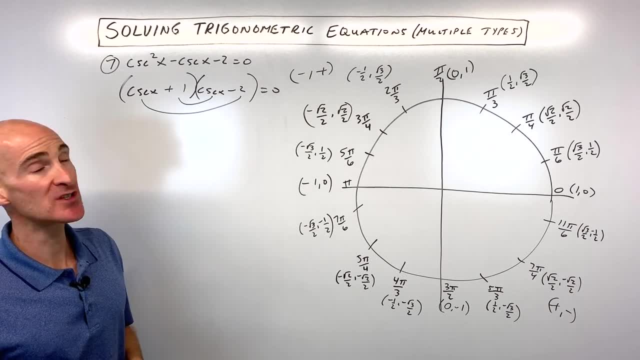 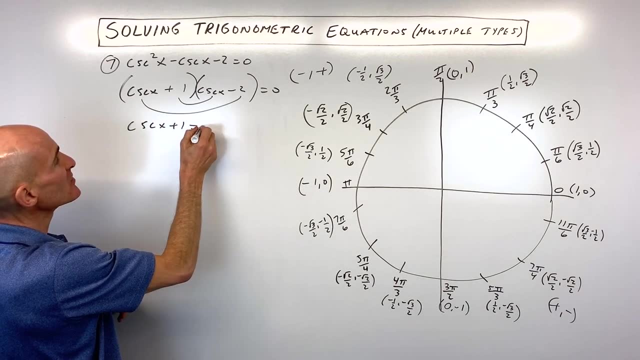 And negative 2 cosecant x Adds up to our middle term Negative 1 cosecant x. So now what I'm going to do Is I'm going to set each factor equal to 0.. Make two little mini equations. So cosecant x plus 1 equals 0. 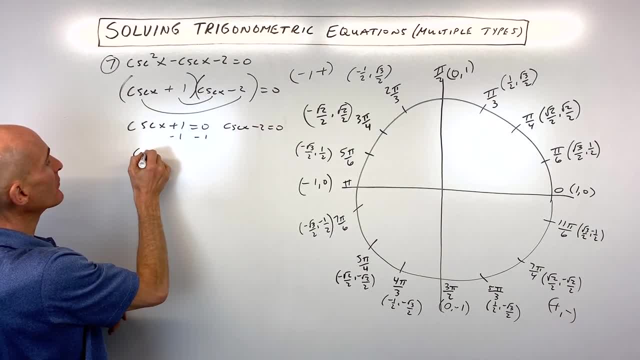 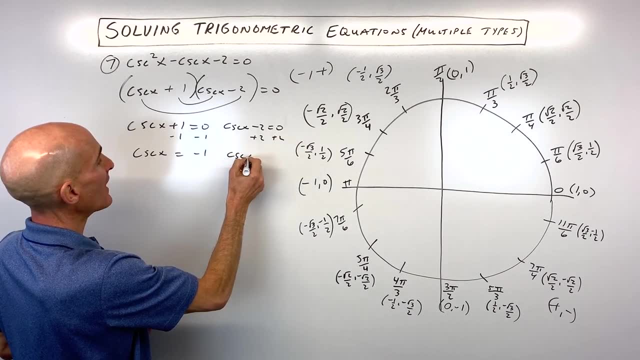 And cosecant x minus 2 equals 0.. Subtract 1 from both sides And we have cosecant x equals negative 1.. Add 2 to both sides And we have cosecant squared x And cosecant squared x equals 2.. 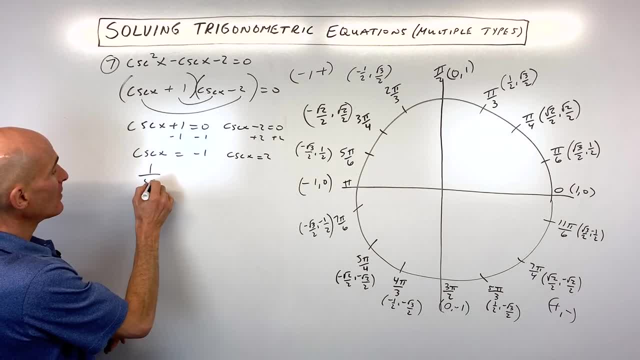 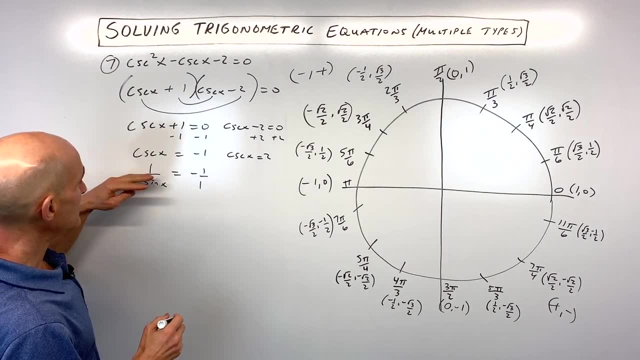 Now remember, Cosecant is really the same as what. 1 over sine And negative 1 can be written as a fraction By writing it over 1.. Anything divided by 1 is itself, If I take the reciprocal of both sides of these. 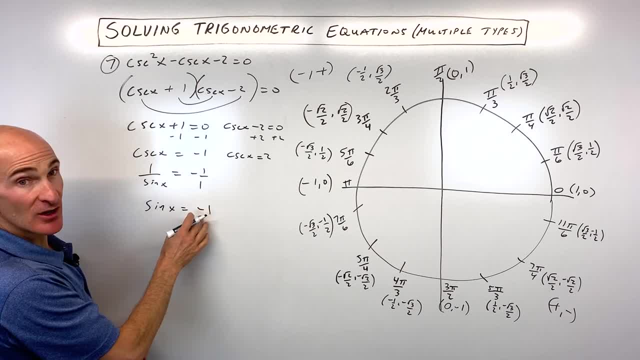 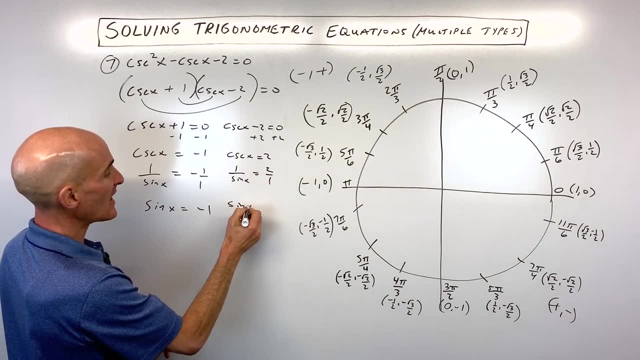 Both sides of the equation here We get. sine of x is equal to. It's still going to be negative 1. Over here, Cosecant of x is 1 over sine of x, Which equals 2 over 1. Negative: 1 half. 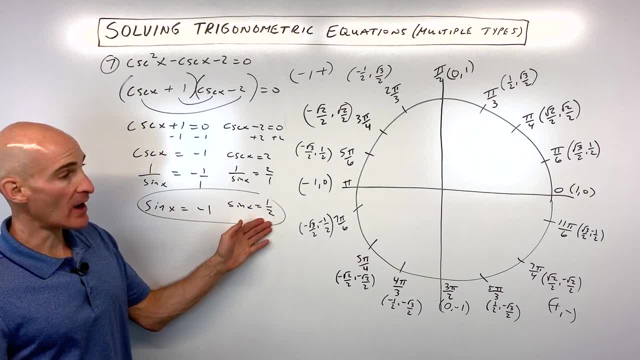 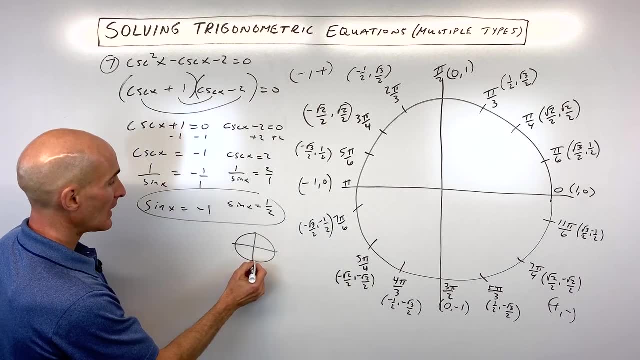 So what we have to do now Is figure out on the unit circle Where is sine equal to negative 1 or a half. So let's take a look. It looks like sine is going to be negative 1 down here At 3 pi over 2.. 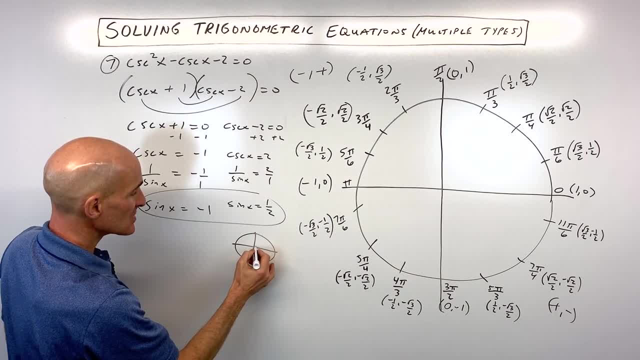 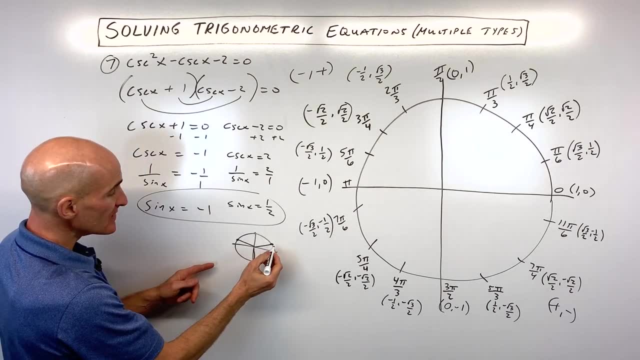 And it looks like sine is going to be a half Over here at pi over 6. And 5 pi over 6.. So right there And right there. Now, if you look closely, It looks like these are actually 2 pi over 3 radians apart. 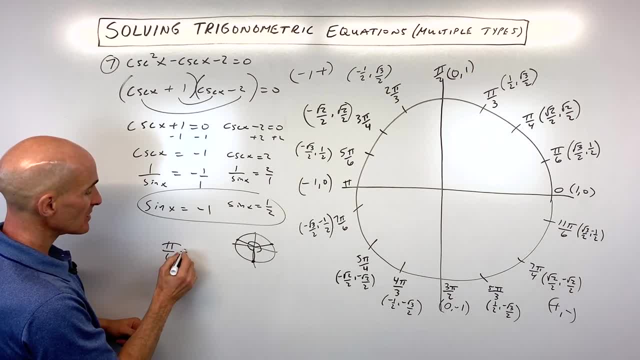 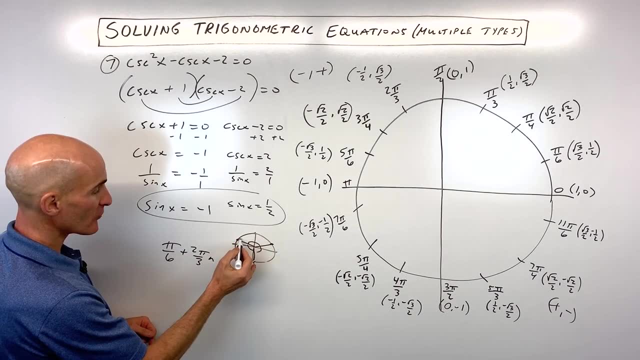 So what we can do is we can group these together. We can start off at pi over 6.. Okay, right here. And what we're going to do is we're going to add 2 pi over 3 n. So if I add 2 pi over 3 once, 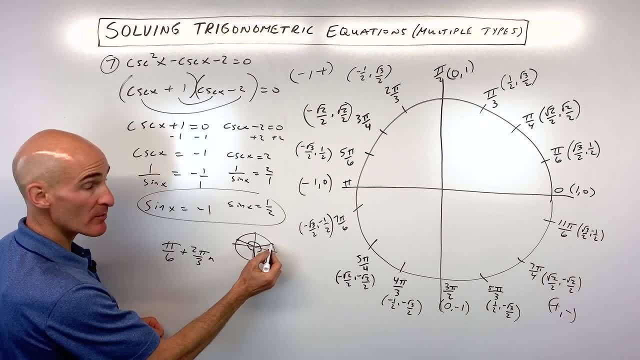 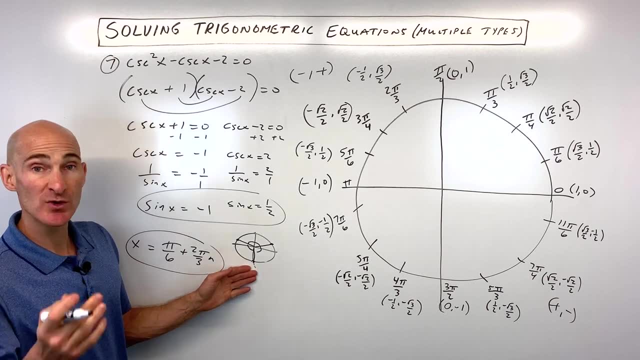 I get to this angle. If I add 2 pi over 3, I get to this angle: Another 2 pi over 3, back to where we started Etc. So that's what x equals as our general solution If we just want to answer the question between 0 and 2 pi. 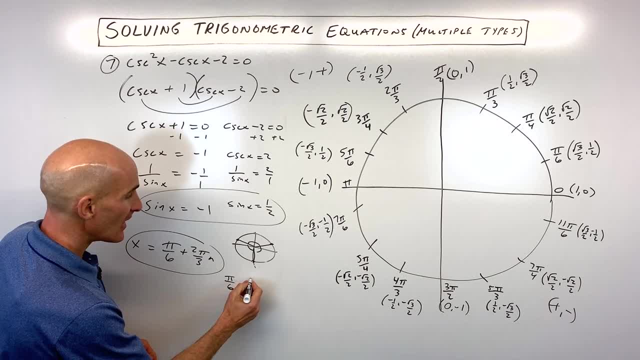 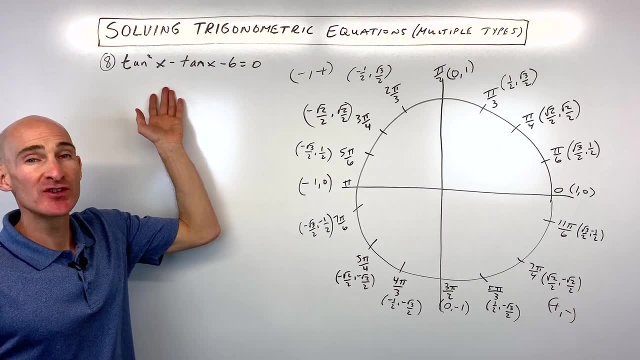 You just list these individually: Pi over 6.. What do we say? 5 pi over 6 and 3 pi over 2.. And you got it Okay. last problem, number 8.. See if you can do this one on your own. 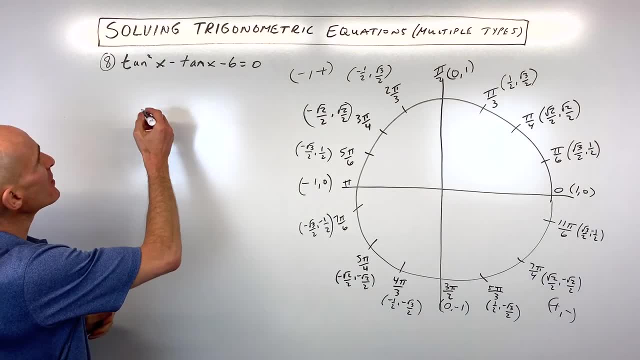 We've got tangent squared of x minus tangent of x minus 6 equals 0.. So what I'm going to do here on this one Is I'm going to factor it Into 2 binomials. We have tangent of x. 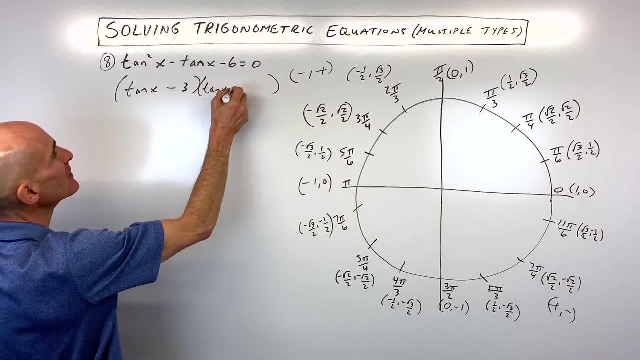 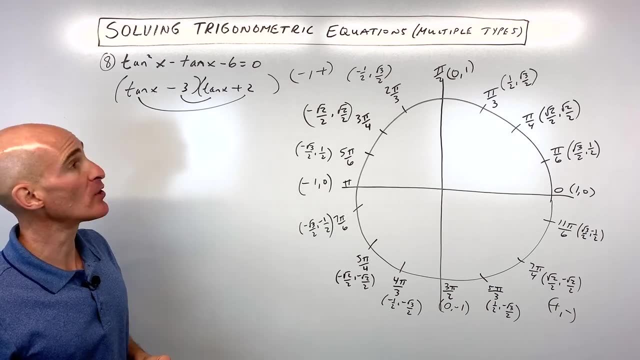 Times tangent of x gives us tangent squared And negative 3. Times positive 2 gives us negative 6. Negative: 3 tangent x And positive 2 tangent x And negative 1 tangent x Equals 0.. So what we're going to do is set each factor equal to 0.. 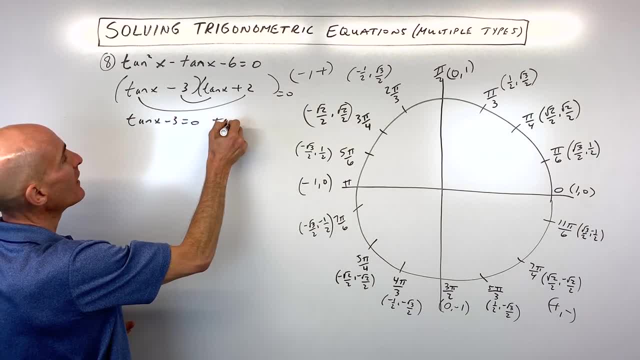 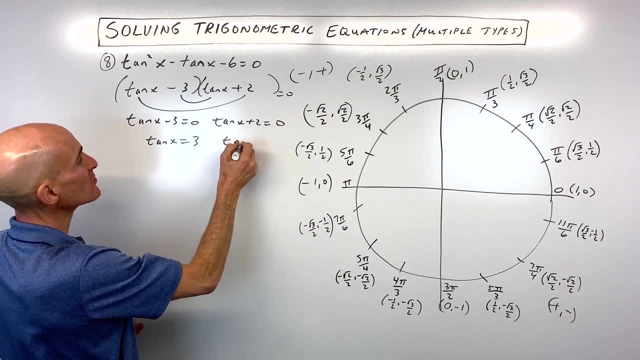 And solve. So we have: tangent x minus 3 equals 0.. And tangent x plus 2 equals 0.. If we add 3 to both sides, We get tangent of x equals 3.. If we subtract 2 from both sides, 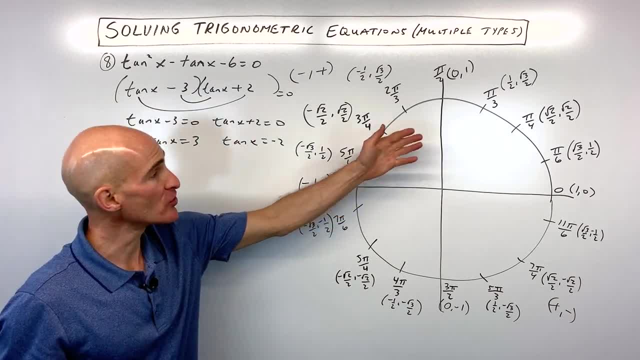 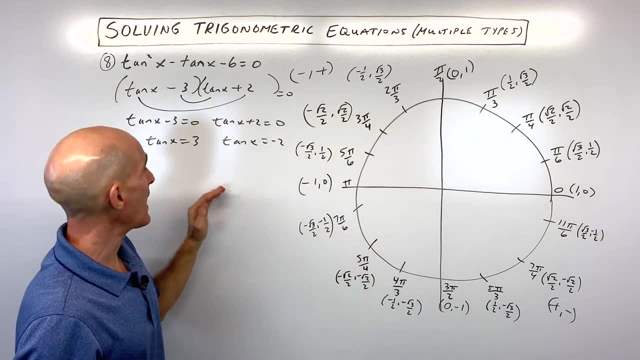 We get: tangent of x equals negative 2. Now on the unit circle There's no location where tangent is equal to 3 or negative 2. With the angles that we know. So we're going to have to go to our calculator. 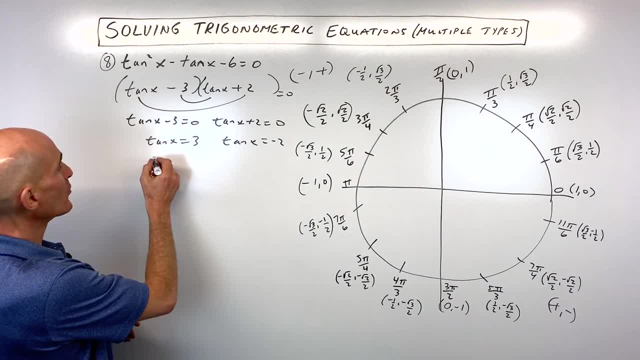 So if you put your mode into radians, And what you're going to want to do Is you're going to want to do the tangent inverse of 3.. And same thing here: You're going to want to do the tangent inverse of negative 2.. 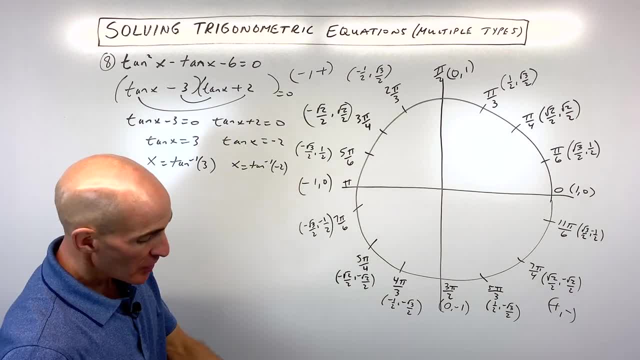 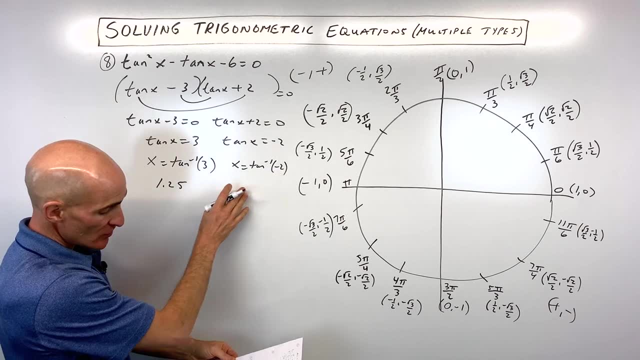 Now, if you do that- I did that earlier here- You're going to get: Tangent inverse of 3 is going to come out to 1.25 radians. Tangent inverse of negative 2. Is going to come out to. 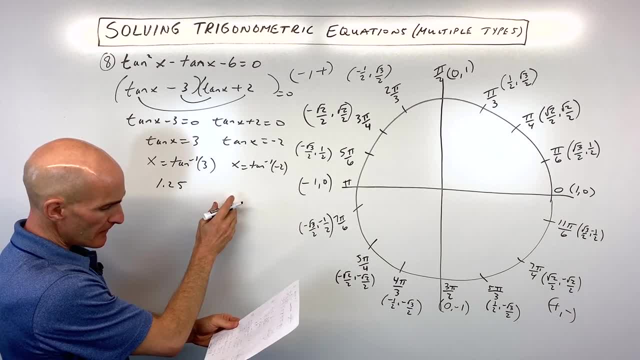 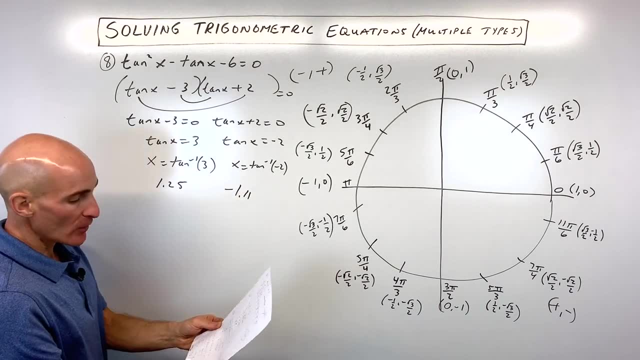 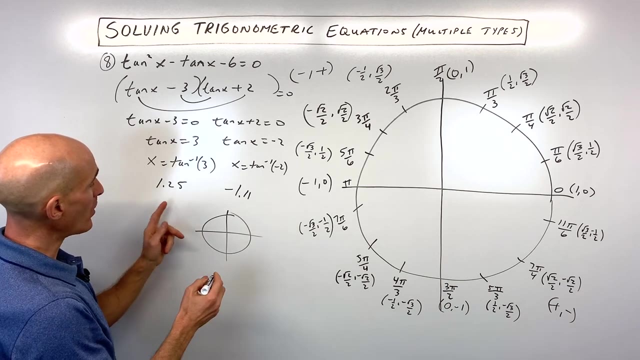 Let's see. This came out to Negative 1.25. And negative 1.11. Radians. Okay, so now what you want to do Is you want to Draw this on the Unit circle here. Now, 1.25 is right about here. 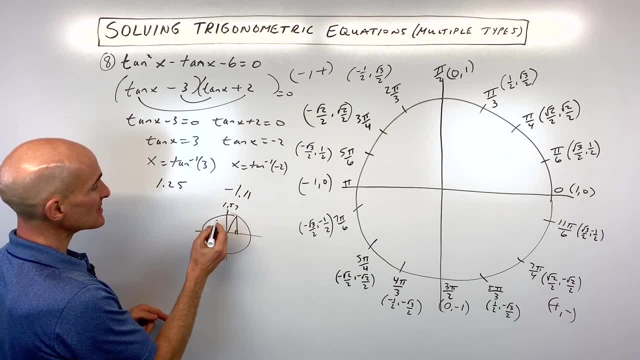 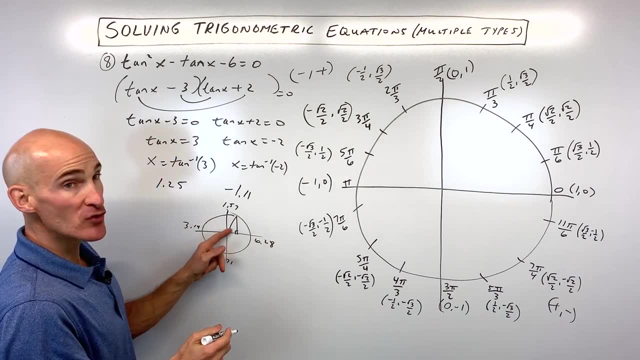 Okay, because at pi over 2. This is like 1.57.. 3.14., 4.71 and 6.28.. So we're here in the first quadrant With the 1.25. But where else is tangent positive? 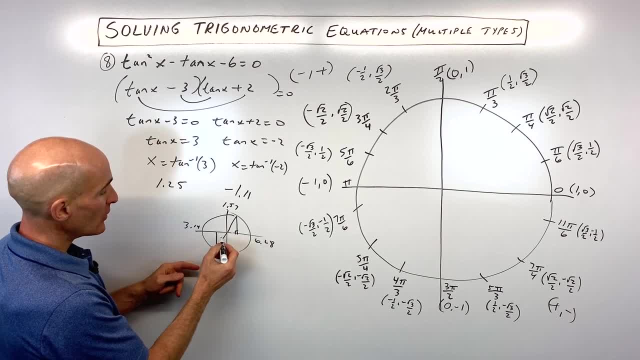 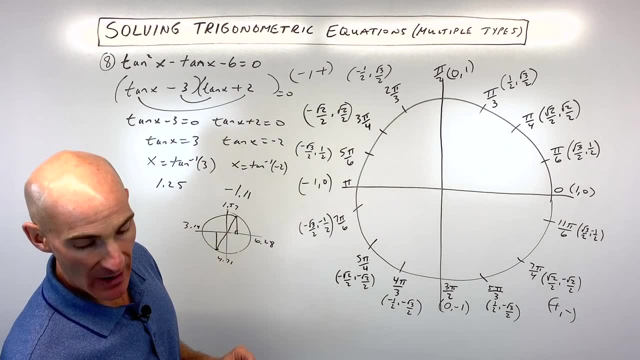 Well, it's also positive over here In the third quadrant, And the way that I can get this other angle over here Is by adding pi. So if I add pi to 1.25.. Okay, remember pi is 3.14.. 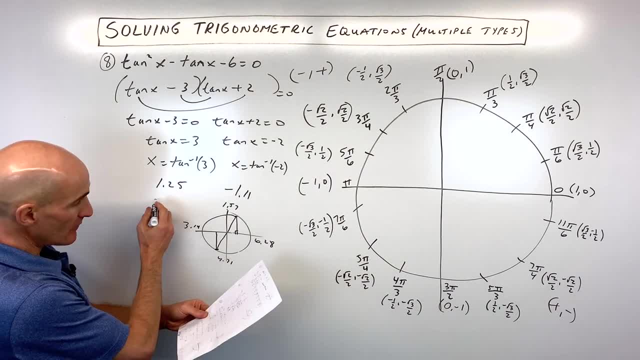 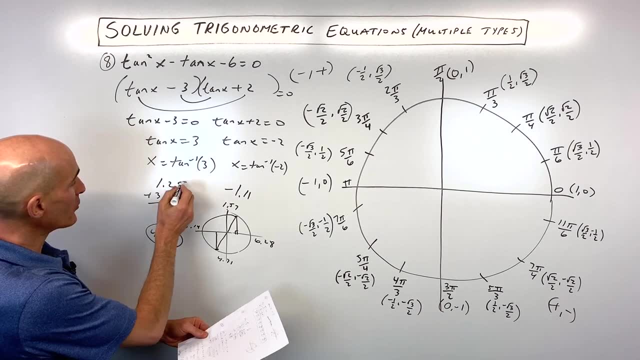 We're going to get Approximately. what is that? Let's see. Plus 3.14.. We're getting 4.39.. So far we have 4.39.. 1.25.. Over here we have tangent inverse of negative 2.. 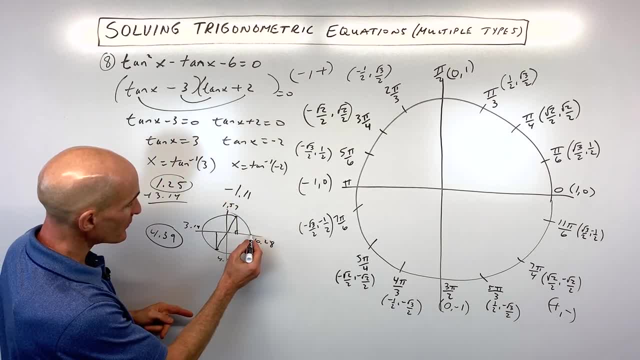 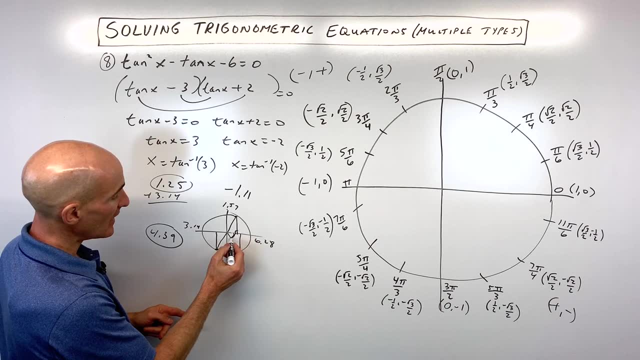 Is negative 1.11.. Now, where is negative 1.11?? We're going clockwise. It's going to be somewhere over here In the fourth quadrant. Okay, so negative 1.11.. Now, if we add 6.28, which is 2 pi, 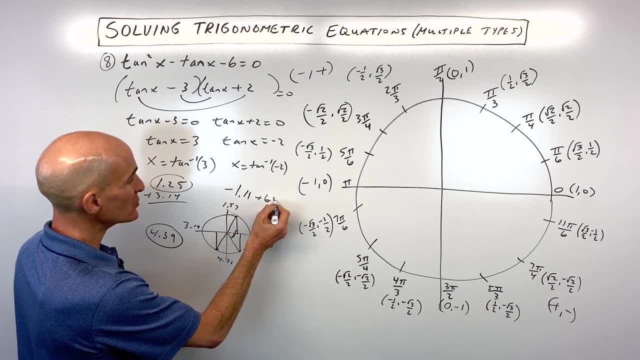 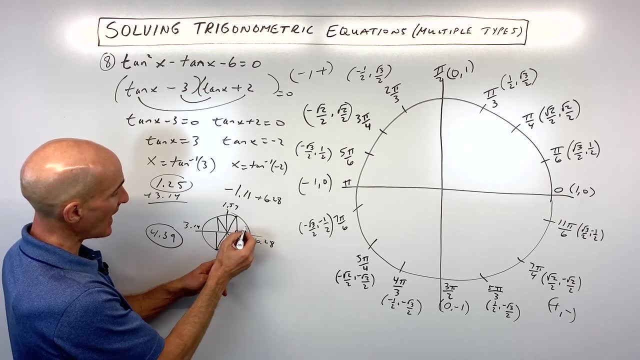 We can get this as a positive angle. Okay, so plus 6.28. Or we can also See tangent is going to be negative 2 over here In the second quadrant. So if I was to add 3.14. That would give us this angle here.